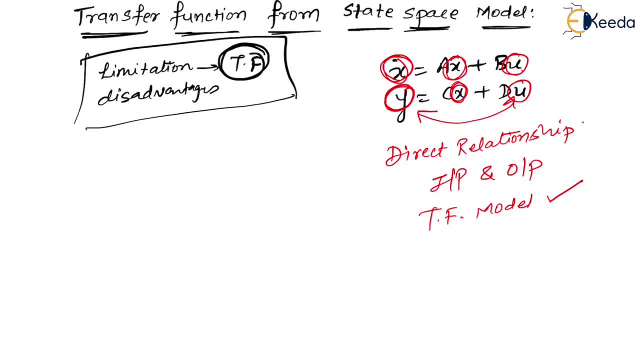 I will give you one very, very practical example in your life, In your student life also. you may think of: See here, Let me consider this is you right Now. let me consider: this is your crush, This is you right Now. your crush has a friend. Let us say this is friend. 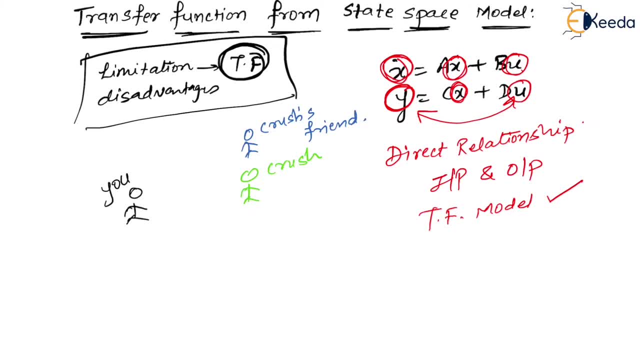 Right. See, here You want to approach. This is you. You want to approach your crush, right? Yes, But you go via this friend of hers to her. Am I right? Most of the cases, people you know have this tendency: They, rather than approaching their crush, they actually go through the crush's friend, right? 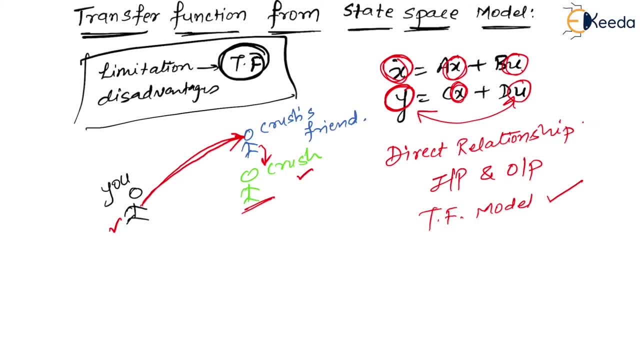 So is it direct or indirect way? Yes, Definitely this is going to be indirect way. If you think of that, this is input, and if you think of this as output, then yes, Definitely, this is indirect way, because you are not directly approaching her. You're not directly approaching her, You are approaching her or him. 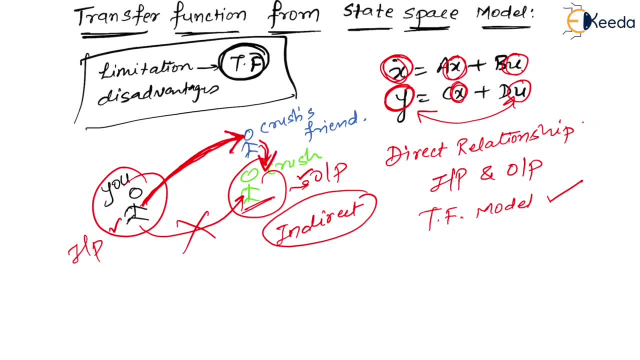 through her friend and you are going to her, Am I right? Yes, So this is called as indirect way, but at the end, if you see, you both need to be together, no, at the end you both need to be together. you both need to be together, right you? 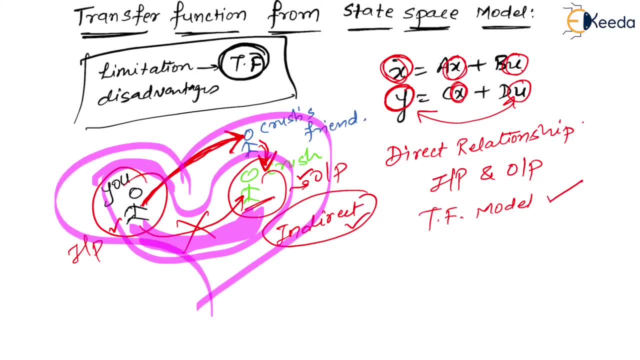 both need to be together. so, in order to do that, you need to approach, approach your crush directly. you need to approach your crush directly, am i right? yes, so see here, even the same way in our systems as well. in our systems as well, you need transfer function model, because you have to use them. you need to have this direct. 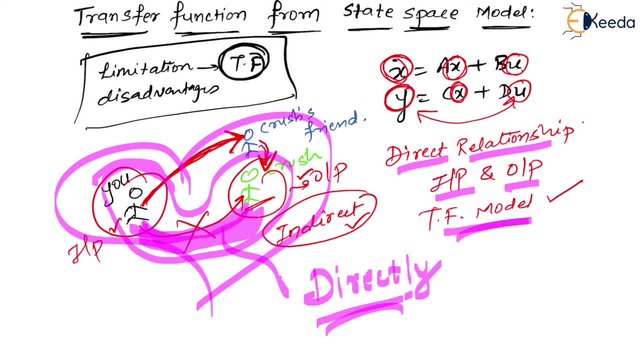 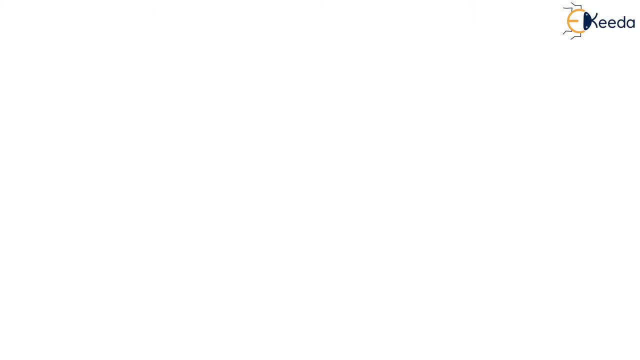 relationship between the input and output. that is the only reason. that's it now. see here, yes. so now let us start with the thing that you know: yes, we have got. this states-based model is not equal to a stars B you, yes, and we know that y is. 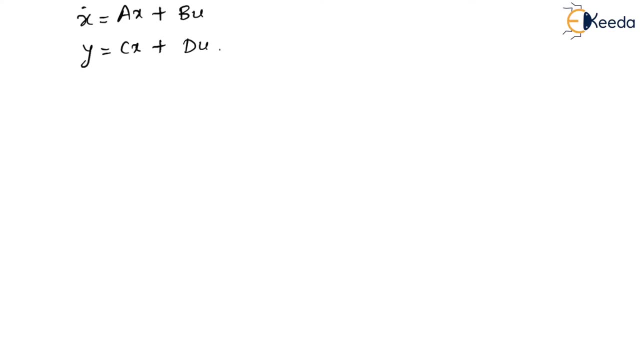 equal to phase 2 g. so this is what we know right now. this is what is given to us. this is what is given to us right now. you need to find transfer, transpose function. all this number means our aim is to find the transfer function. Now you please tell me what is the transfer function? 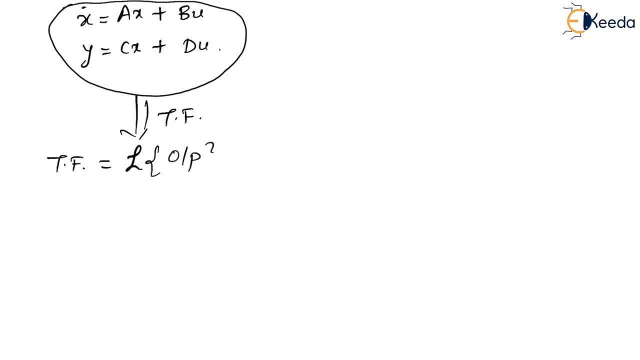 Yes, transfer function is nothing but Laplace of output upon Laplace transform of input, keeping initial conditions, initial conditions, as 0. That is what we know So now, which means that in order to have transfer function, you need to firstly have Laplace transform, or not. 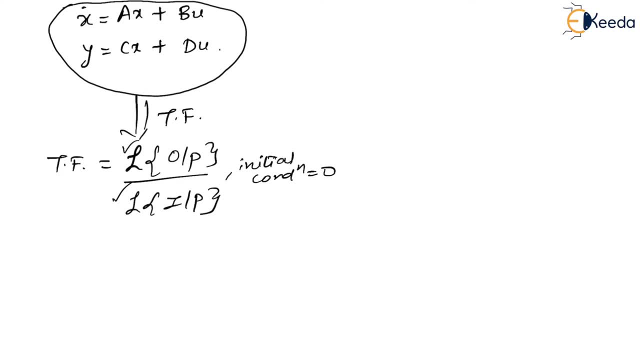 Yes, definitely. So let us try to apply this Laplace transform to our state space equations. Let me call this first equation as 1 and let me call this equation as 2.. Is that fine? Yes, no problem. Now let us apply Laplace transform. 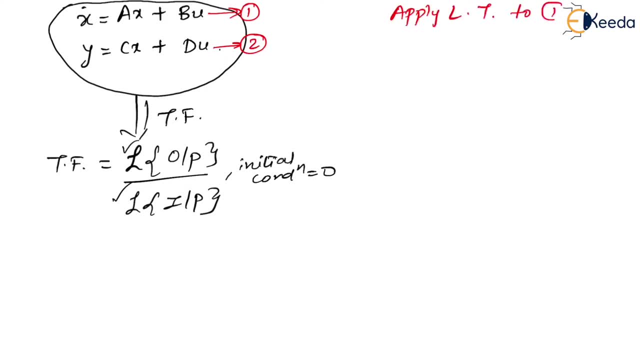 Let us apply Laplace transform LT to first equation. If you apply it to the first equation, what you have got is: yes, you have got Laplace of something LHS into Laplace of some RHS right Inside this LSH. yes, definitely, you are going to have x dot. 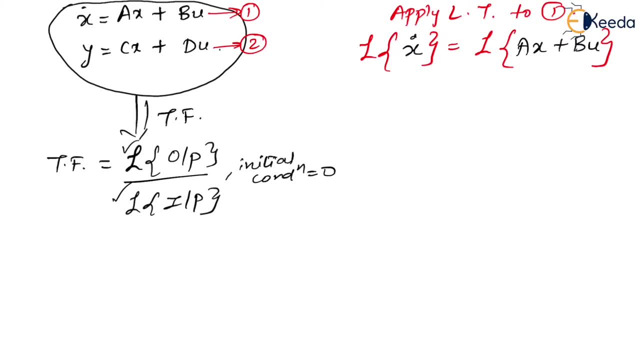 and here you are going to have x dot plus BU, Right, yes, now, if you just see here, this is x dot, right? What do we mean by x dot? X dot is nothing but first derivative of x, Am I right? 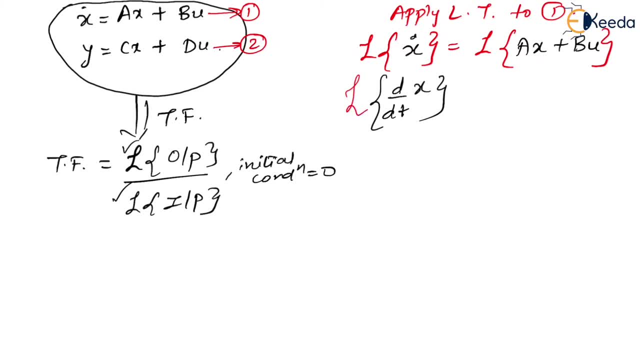 And you need to find Laplace transform of the same. So yes, if you know the property, let me just take the property here down. See here you know the property. If x of t, Laplace transform of x of t is, let us say, x of s, 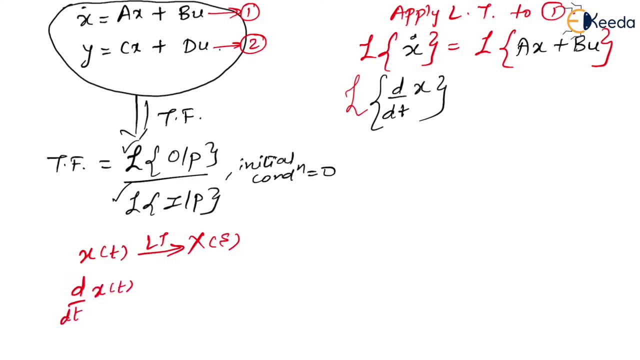 Then Laplace transform of dy dt of x of t is going to be what s into x of s minus x of 0. That is what we know, right. This is from property of derivative, property of differentiation, differentiation in time, property right. 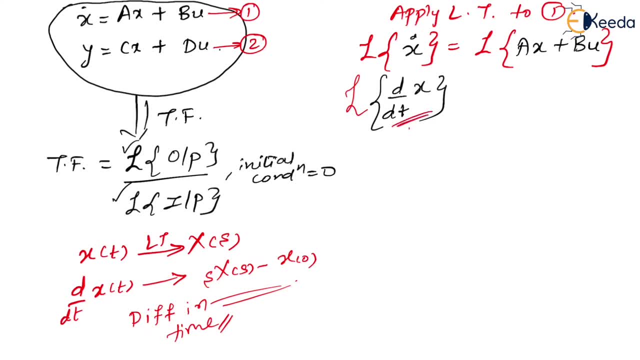 This is what we know. So, yes, if it is dy dt of x of t, then let us just simply replace, Let us just simply find the Laplace. So we just have this Laplace transform as s into x of s. 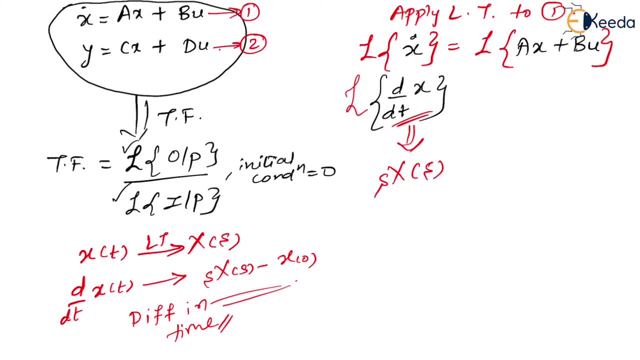 Now you may ask me, sir, yes, if it is x into x of s, but now why you are not considering x of 0 minus x of 0?? By the way, this x is small, right? This x is small, which means this x is in time. 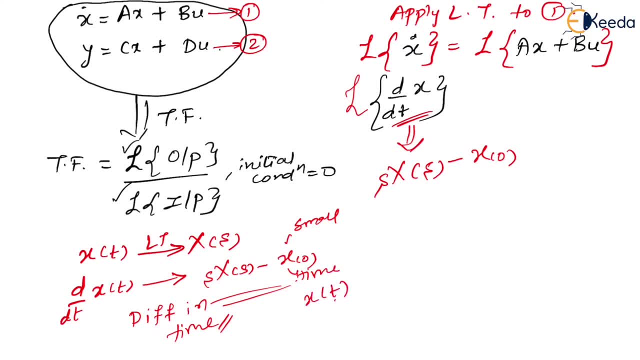 Means basically wherever in x of t you have to this small x of t, because, see, capital is going to be for s right. So if you have this small one, so in place of t you need to put 0.. 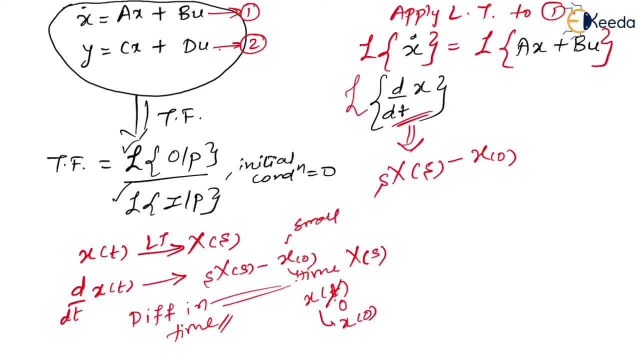 Then you get this x of 0. That is what we know. But then are we interested in it? Let us see No, Why? Because we know that initial conditions are going to be 0. The moment we say that initial conditions are 0, so x of 0 is going to be 0. 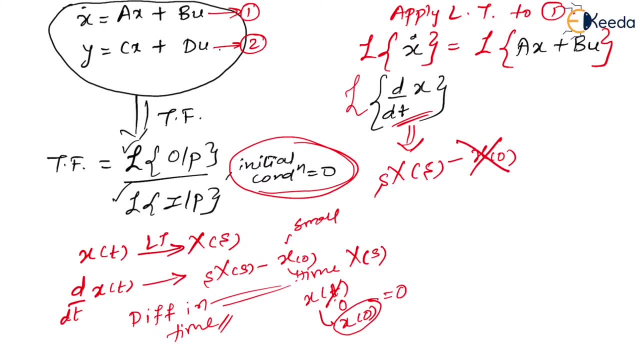 If x of 0 is going to be 0, then this term need not be considered, So let me just erase it Right. Yes, Now equal to. if you think of s, Now we know that Laplace is a linear operator. 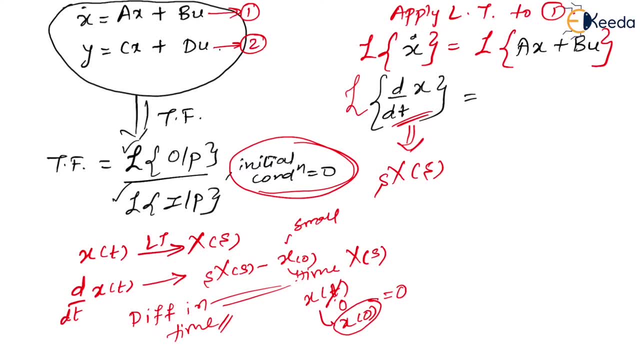 Linear operator. Linear operator In the sense means if I am applying Laplace transform to ax plus bu, which means it will get separated Means Laplace of ax plus Laplace transform of bu. That is what can happen, Right. 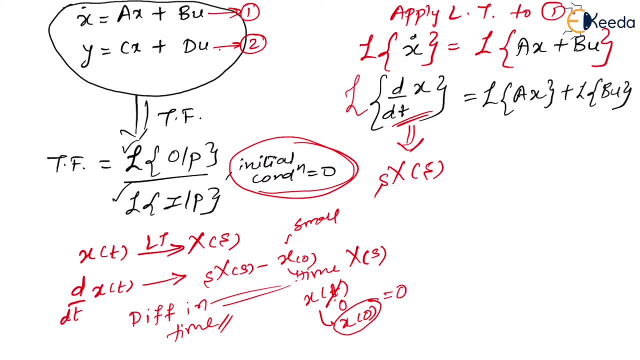 So if I think of here, then this is going to be this: a will come out, So it becomes a into Laplace of x of t is just going to be x of s plus yes, What is this? bu? So it is going to be b into u of s. 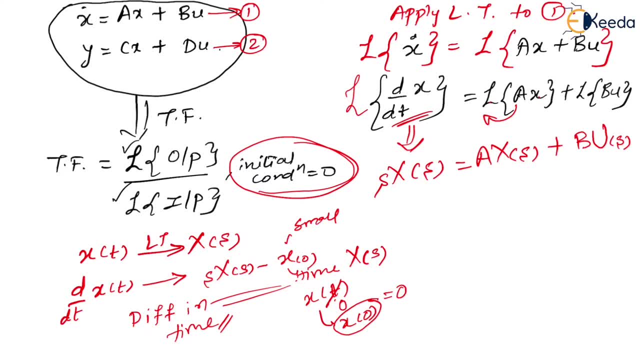 This becomes capital U. By the way, this is not u of t. Most of the time people say that, sir, no, this is input. No, this input is u of t. See, u of t is a step signal, we know. 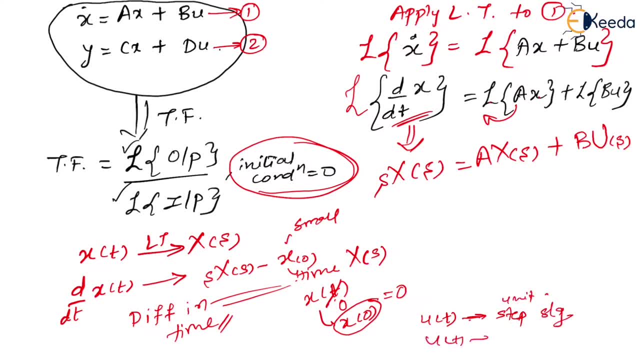 u of t is a unit step signal Right, But here u of t means input In our state space thing. here u of t means it is the input. You need to understand this. Keep that in mind. Here u is nothing but input. 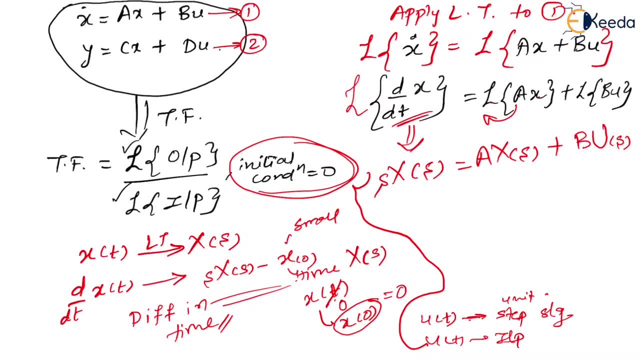 Whereas u of t also means unit step signal, we know, But here u of t, u of t is nothing but the input And that can be again. that can be a step signal, That can be a ramp signal, That can be a parabolic signal. 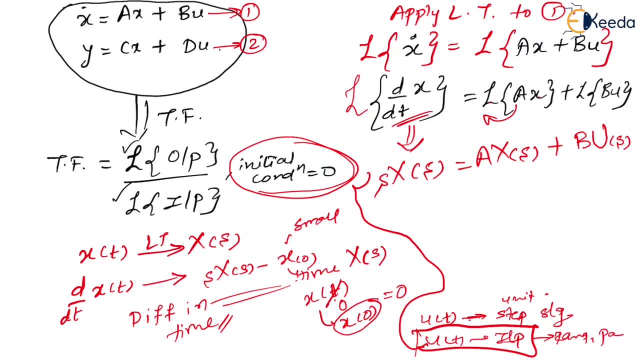 Any signal you want, Right? So this is what is the first equation we have got. So let me just say that this is equation 3.. Let me note it down as equation 3.. Right Now, let us try to do the same with equation 2 and see what happens. 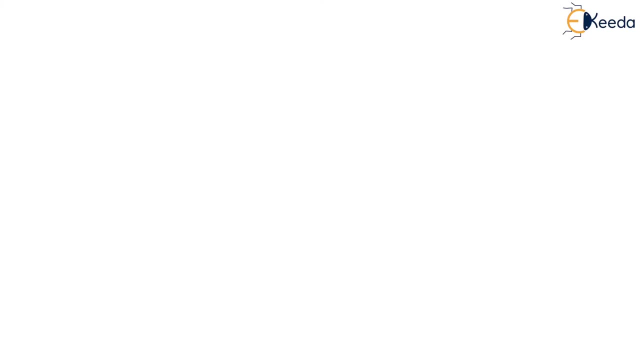 Right, Yes, What was equation 3?? What was equation 3?? Yes, it was y equal to cx plus du. Right? So let us apply Laplace transform to this also, So this becomes Laplace of this into Laplace of this. 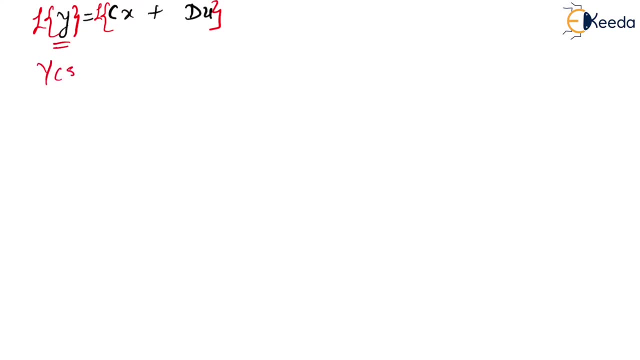 Right, So it is going to be Laplace of y. right, So it is going to be y of s, which is equal to cx, So c comes out and this is x of s Plus yes, definitely Laplace of d. 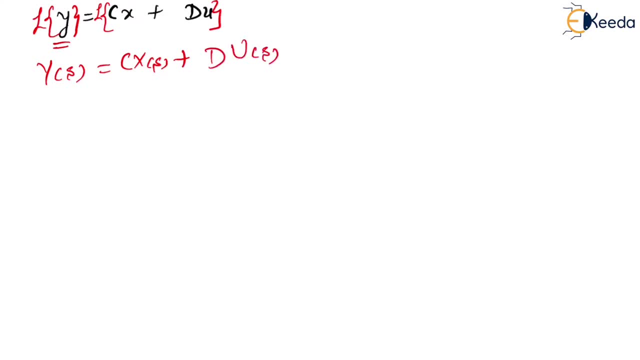 So it will be d into u of s. This is what is there? The same thing, The same thing, Right? So let me call this as equation 4.. Let us call this as equation 4.. Now you have got this y of s right. 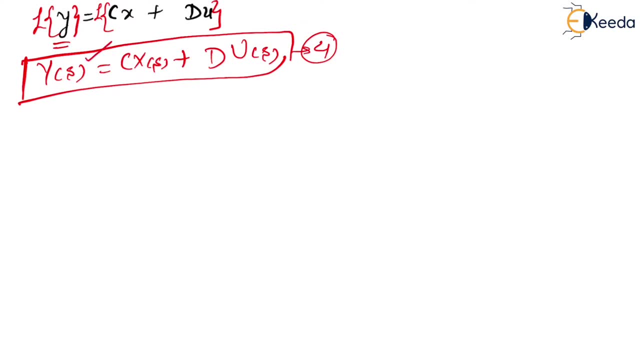 Yes, You have got this y of s And you need x of s also. So x of s is here also And x of s is here also. So basically, yes. So you may say that, yes, this y of s, which is there, is nothing but Laplace of output. 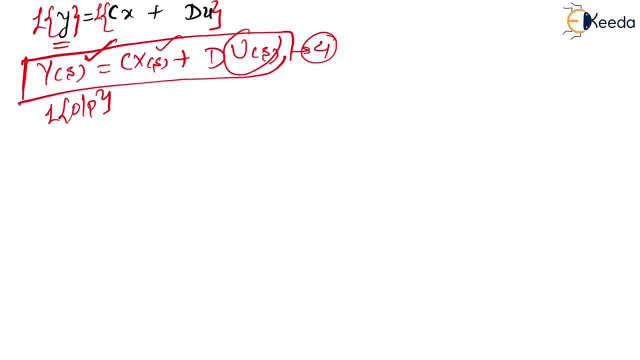 Yes, definitely, it is Laplace of output. we have got, Similarly, if you think of this, u of s also. yes, definitely, it is Laplace of output. So it is going to be Laplace of input, right? Yes, 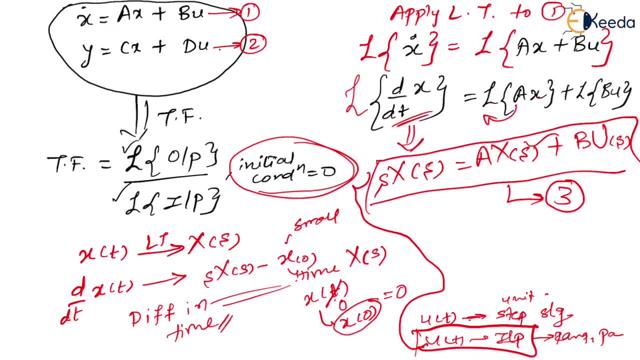 But if you see the same thing we have in equation 3, also In equation 3, if you see same thing we have, This is nothing but Laplace of input. And if you think of yes, input is also there. 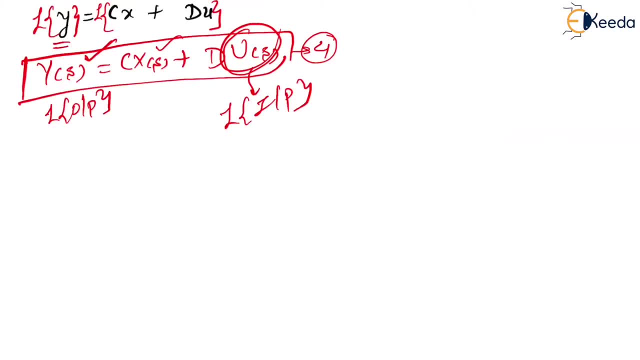 Which means what has to be there. See here itself: if you see you have this Laplace of output available, You have this Laplace of input available, But this x of s is the culprit. So by some means, this term, this term has to be replaced. 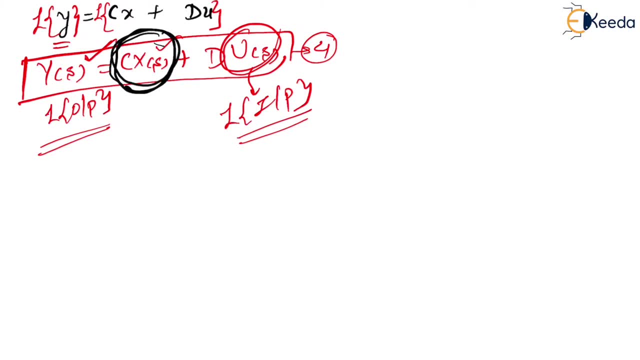 This term has to be replaced, Which means x of s has to be replaced. So how to replace that x of s? For that, let me take help of equation 3.. From equation 3, if you see what we have got from equation 3.. 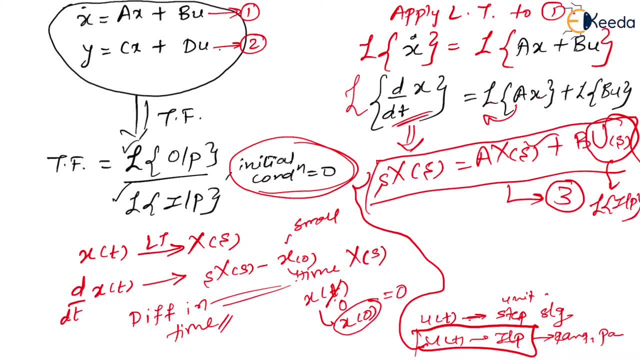 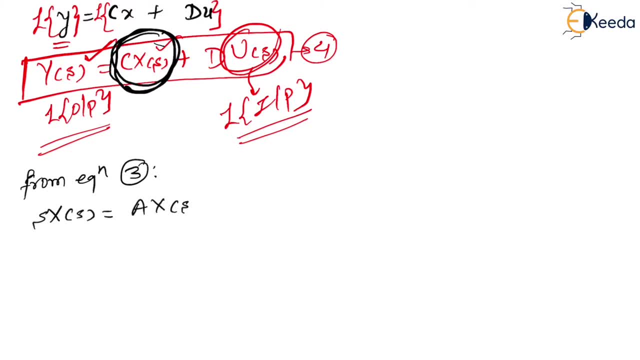 Equation 3 is s into x of s minus a into x of s plus b into u of s. So it is s into x of s. So it is s into x of s minus a into x of s plus b into u of s. 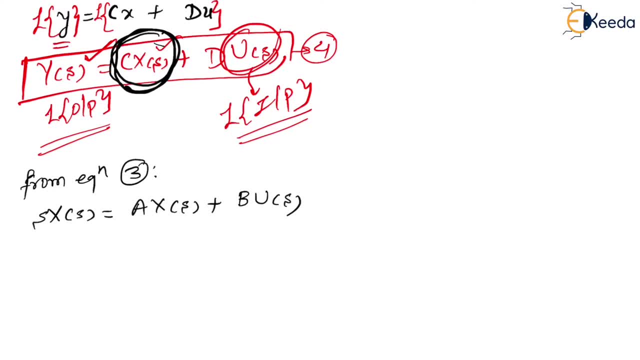 Right Now. what we need to do here is just simply take x of s common In the sense. see, let me take this s into x of s here, Let me take this term to the left, So this becomes minus a, into x of s. 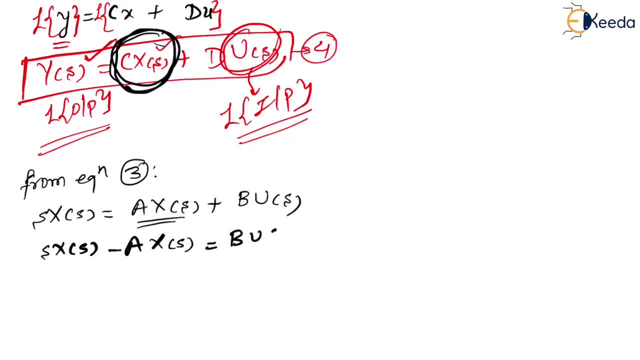 Right, Which is equal to b, into u of s. Yes, perfect, No problem, Right, No problem. Now can I write it as s minus a? If I just think of taking x of s as common. if I take x of s as common. 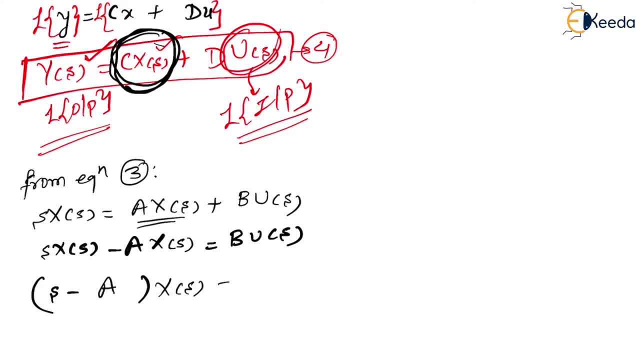 So here I can write, as s minus a is equal to b, into u of s, Capital, U of s. Is it right? Is it right? You please tell me No, Why? Because we know that this x of s, this is the matrix. 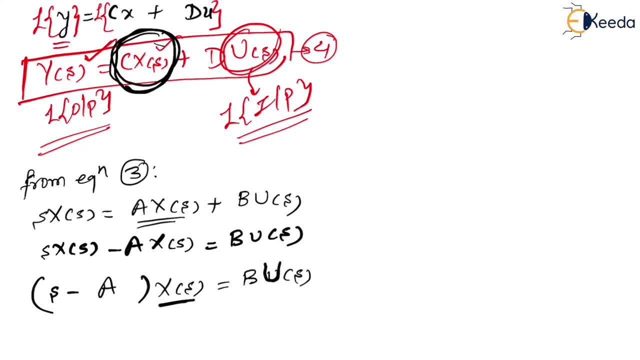 Because this x? we have already seen that x is a vector, u is also a vector, So this cannot happen. So, in order to say that this s- if you just see here, this s, it is just a simple algebraic term. 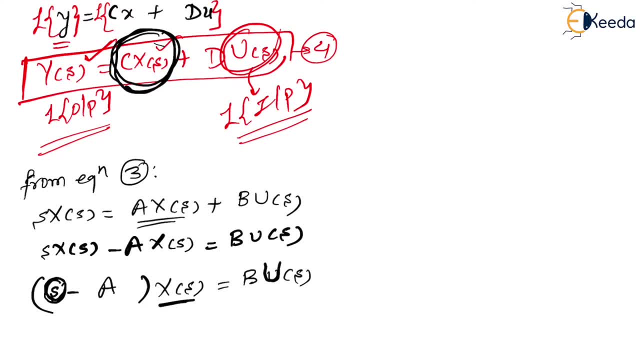 It is just a simple algebraic term. It is not a matrix. This s is not a matrix. If you think of this a, this a is a matrix. This x, this x, is a matrix. If you think of this b, it is a matrix. 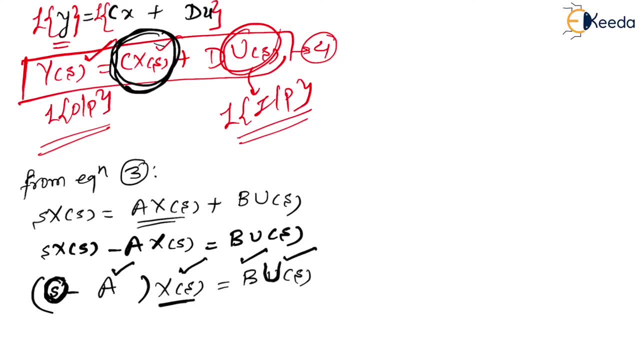 If you think of this u, it is a matrix. But this s is not a matrix. It is the number you can think of. So if you think of s as a number, then it is going to be number minus matrix. Is it possible? number minus matrix? 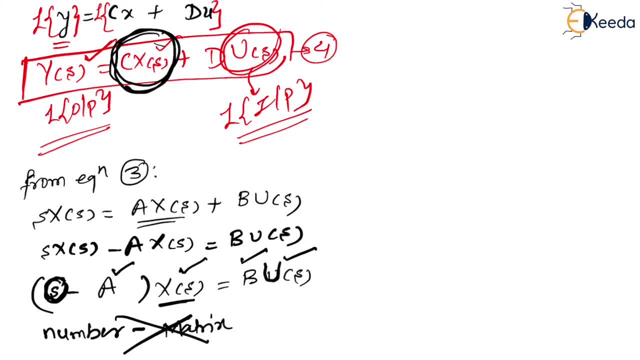 No, it cannot be possible. It is not possible. So, if it is not possible, which means this s has to be converted into matrix. So, to convert this s into matrix, what we do is we simply multiply this s By i. 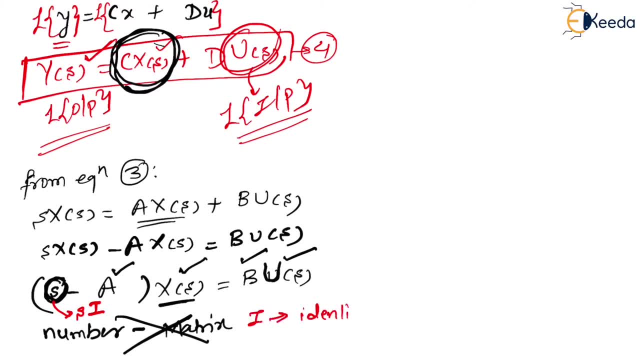 What is i here? Yes, i is going to be identity matrix. i is going to be identity matrix. So if you just see here, yes, Yes, If you just think of so, if I replace this si, so I get s into i minus a into x of s is equal to b into u of s. 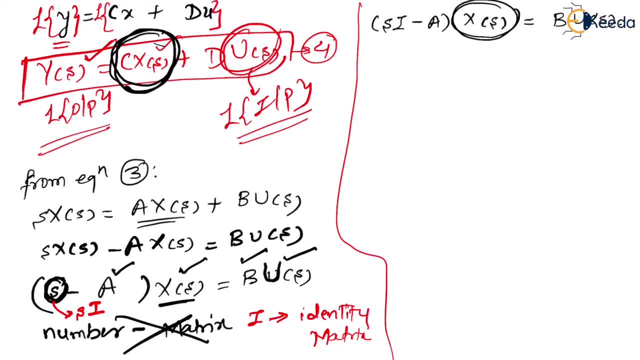 Yes, Now we need x of s on one side, right, Yes, we need x of s on one side. But if you see, yes, now student may say that, sir, it is going to be very, very easy. you know, just keep this x of s here and just divide this one here. 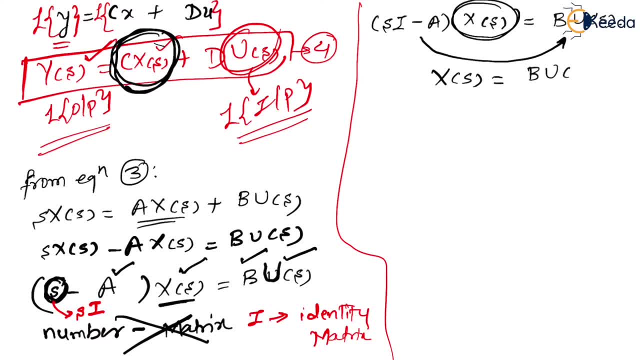 So student may say that, sir, please do it this way, that x of s is equal to b, into u of s upon si minus a. Is it right? No, this cannot be done. Why? Because we know that matrix division. 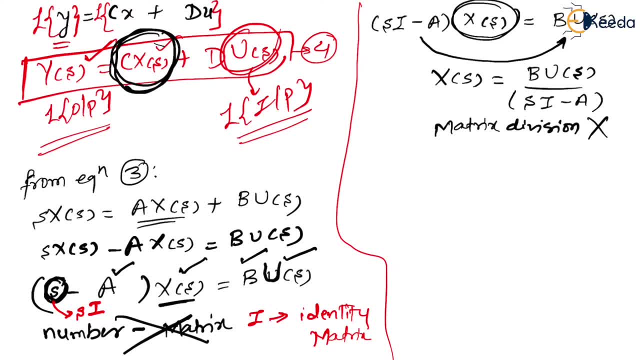 Matrix division Not possible. Matrix division is not possible. So which means, which means this step is not possible, You cannot do this one. If you cannot do this one, then what has to be done in order to keep this x of s on one side? 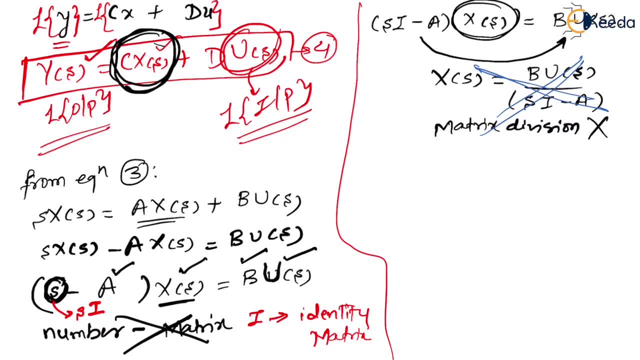 So, in order to keep this x of s on one side, what we can do is we can use left cancellation method, which you have learned in mathematics. Yes, So if you think of left cancellation method, what is there in left cancellation method? 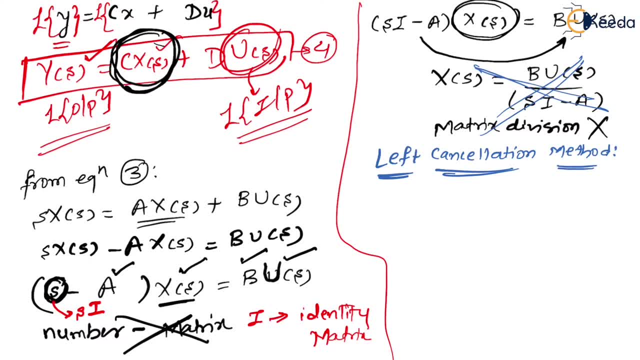 In here what we do is we just pre-multiply by the term which we don't need. We just pre-multiply by the inverse of the term that we don't need: Means. if you see here, here, this is si minus a, is there? 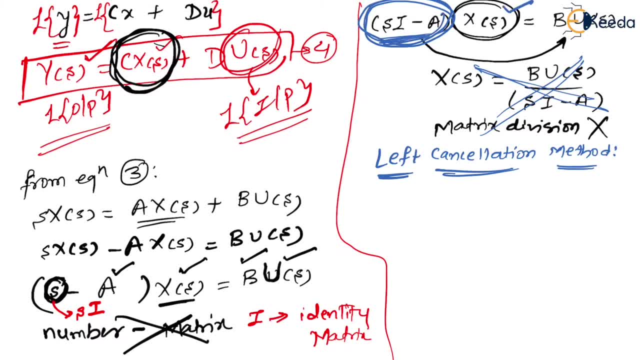 You are not interested in this one. You only want this x of s right. So what you do is you just pre-multiply. pre-multiply by inverse of the term. So let me pre-multiply by si minus a. 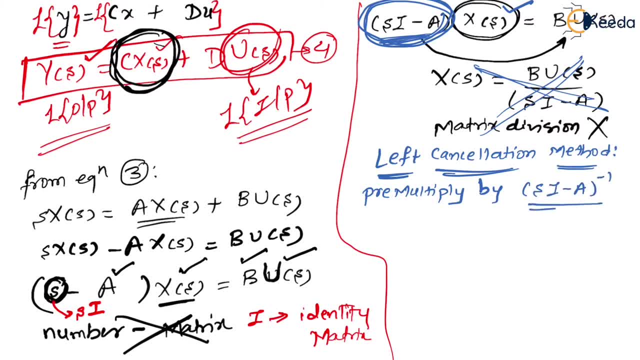 Si minus a inverse. So if I just pre-multiply by si minus a inverse, what do I get here? Yes, I get si minus a inverse and the whole thing repeated. Si minus a into x of s is equal to b into u of s. 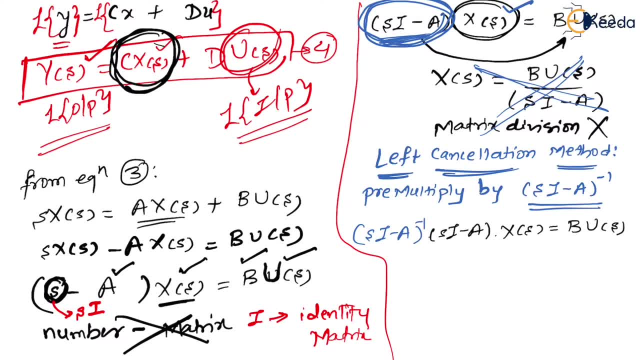 Am I right? Yes, So can it be done on only one side? No, it has to be done on both the sides, which means even on the RHS we have to do the same. So in order, so you need to. so now student may again say: yes, sir, just simply multiply it. 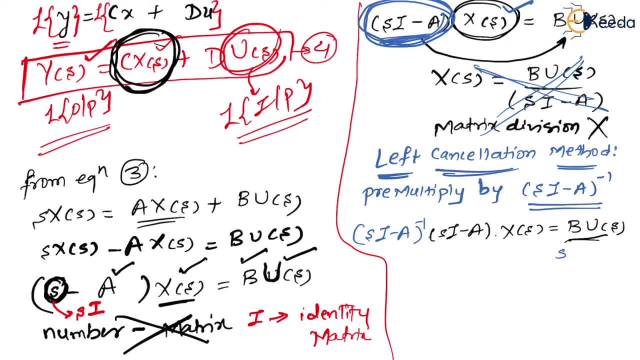 So student may say that: yes, sir, just simply multiply this one as si minus a inverse. also here, also there is no problem. Is it right? No, it is wrong, You are pre-multiplying here. or you can say: you are multiplying from left here. 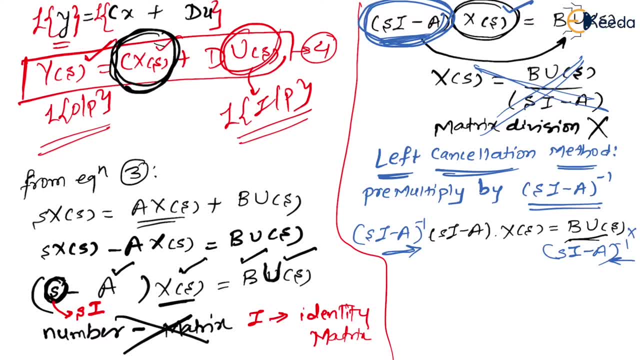 and here you are multiplying from right. It is not possible. If you are pre-multiplying on one side, then on the second side also you need to pre-multiply. So you cannot do this one. So what you have to do is I will erase this and write. 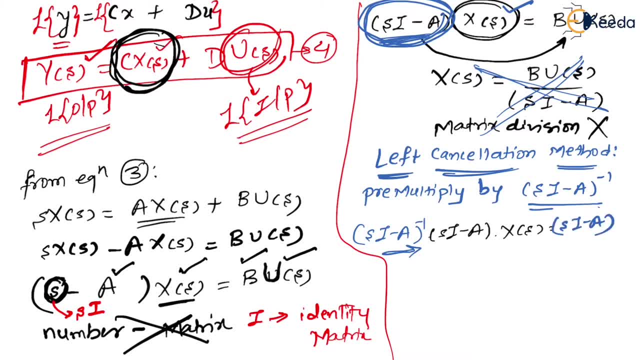 Yes, So you need to have this si minus a inverse here, right multiplied with b into u of s. That is what was there? this b into u of s. Same thing has to be taken here, right? So if you just see here, 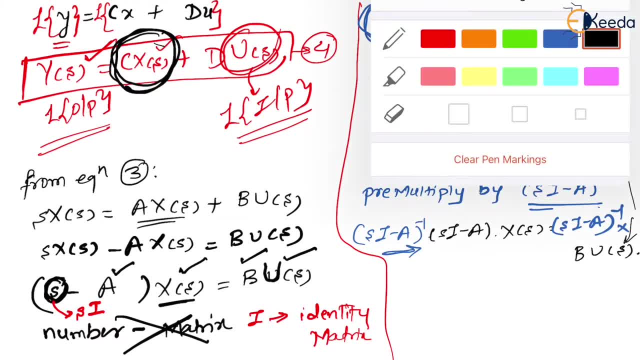 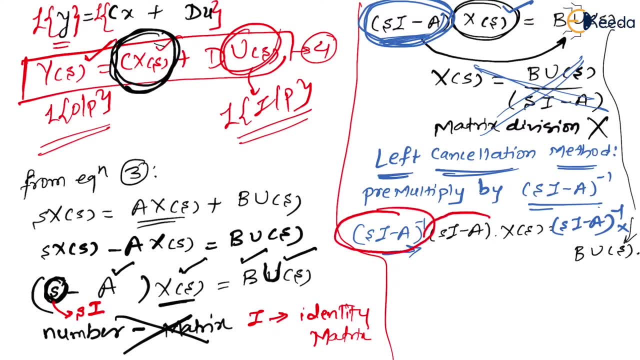 yes, this is. do you agree with me that? do you agree with me that this is the matrix? yes, Do you agree with me that this is the same matrix? yes, Means whatever this matrix is, whatever this matrix is, the inverse of this matrix is here, right, 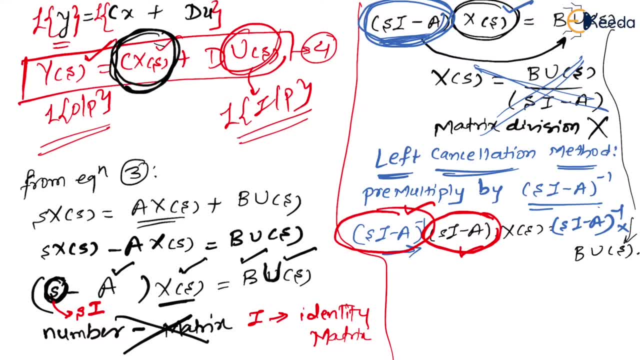 So matrix into its inverse is going to be the same thing. It is going to be i, which is 1.. So I will just have this x of s now here. So I will just have x of s here Which is equal to yes, definitely si minus a inverse si minus a inverse into b, into u of s. 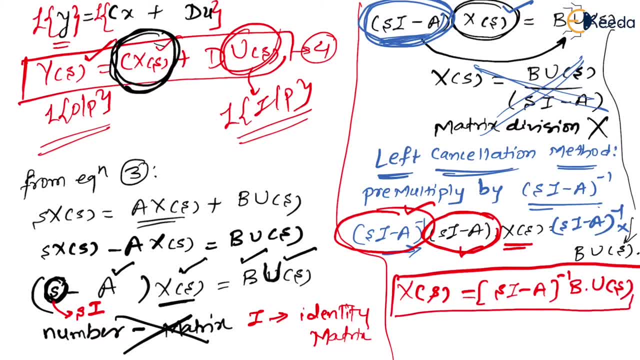 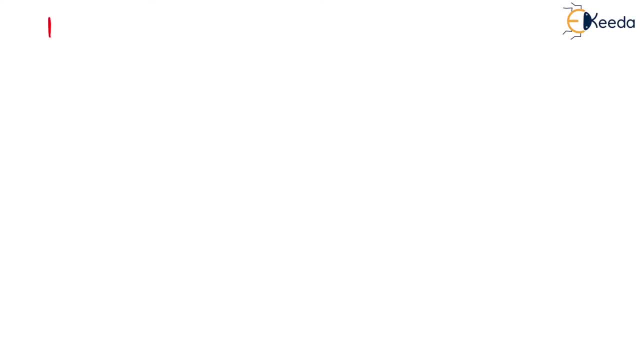 So now, since we have got the value of x of s, we just need to simply replace it in equation 4.. So let me call this as equation 5.. Now let me put equation 5 in equation 4 and let us see what happens. 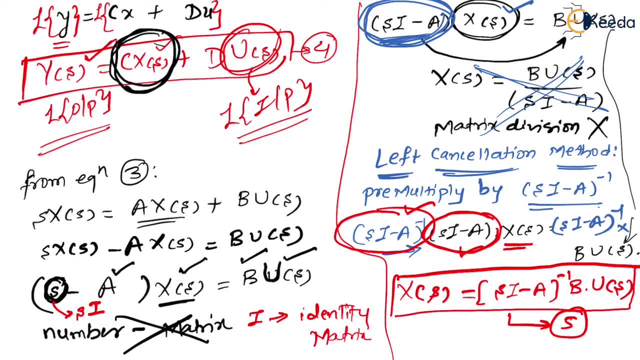 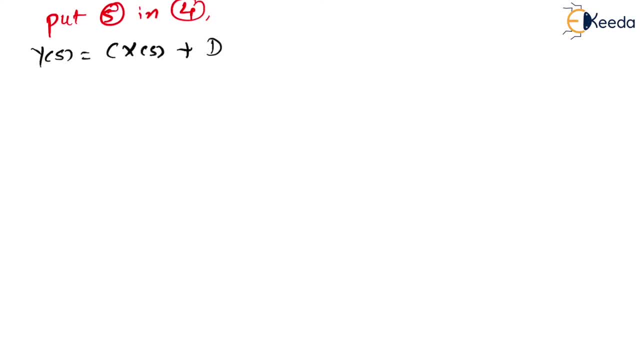 If you see here, equation 4 is what y of s equal to c into x of s. So y of s is equal to c into x of s, plus d into u of s. am I right? Yes, So you need to apply. you need to just simply replace x of s by the value it has. 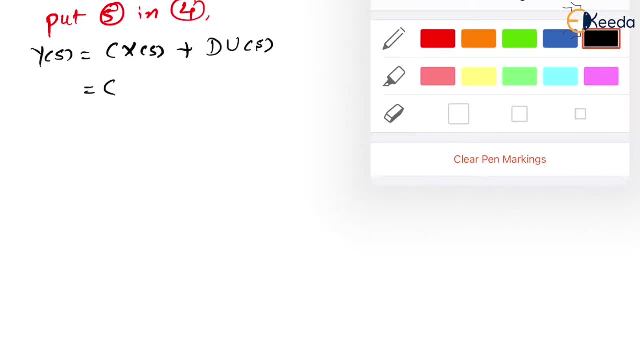 So let me have this c into yes, x of s. So let me replace this x of s term here. So in x of s what we have is yes, x of s is nothing but equation 5.. 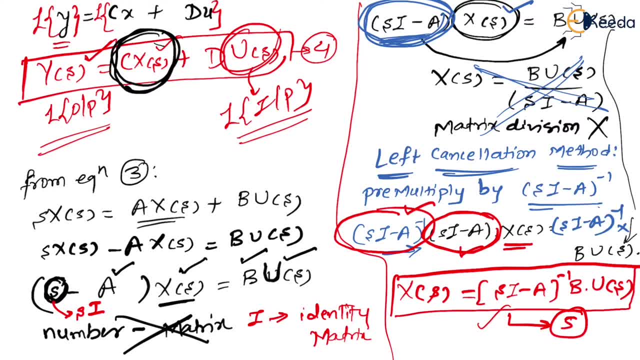 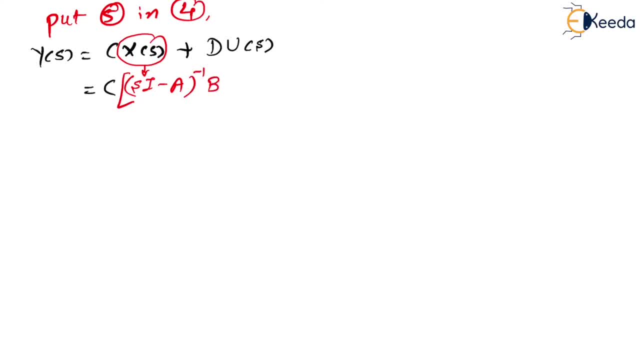 So it is this one: si minus a inverse into b, into u of s. So it is going to be si minus a inverse into b, into u of s, into u of s. right, This is what is the thing, plus the remaining stuff, plus d, into u of s. 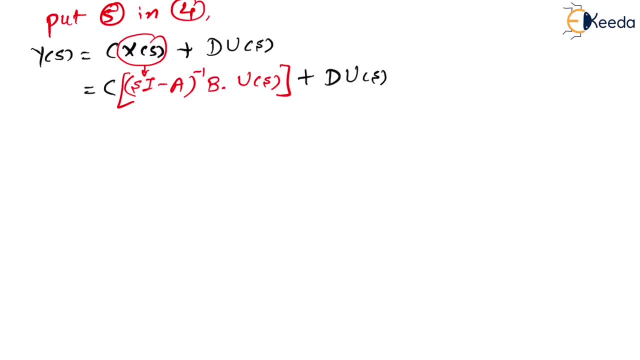 Is it all right? Yes, Now, if we, just If we just observe here you have this u of s and this u of s as common and they are added. So let me just take u of s outside, Let me just take u of s common from both these terms, because this is one term. 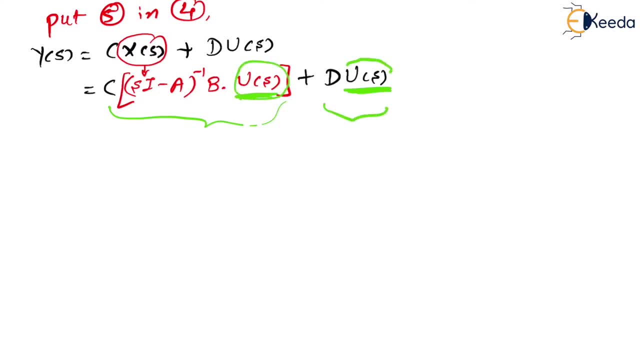 This is another term And out of this, this u of s and this u of s are going to be same, So let me just take them out. So if I take them out, so what do I get here? Yes, 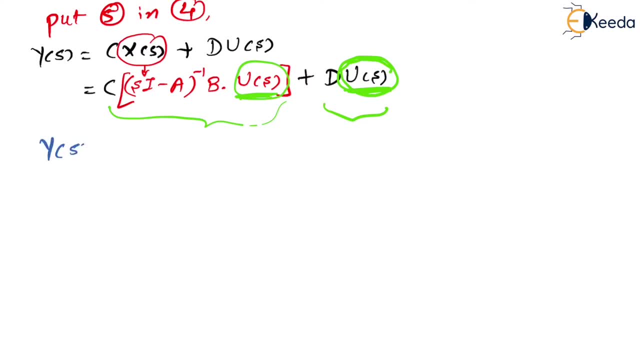 So I get. So inside I get, Let's see y of s equal to Inside. I get c into si minus a, inverse into b plus d. This d should also come right, And the whole thing, the whole thing which is there, that is going to be multiplied by: 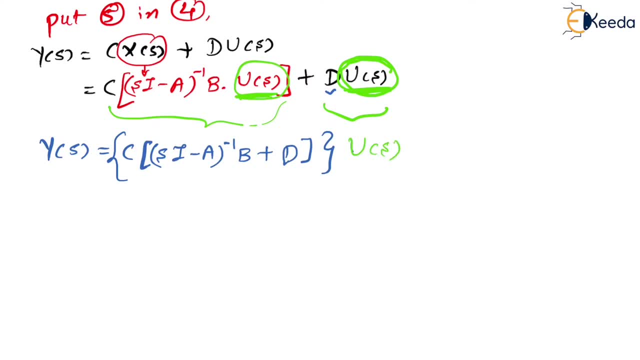 It is going to be multiplied by u of s, Am I right? Yes, So now you have got this input, u of s, and you have got this output, So you can just take it this way. So now, we shouldn't do it this way? 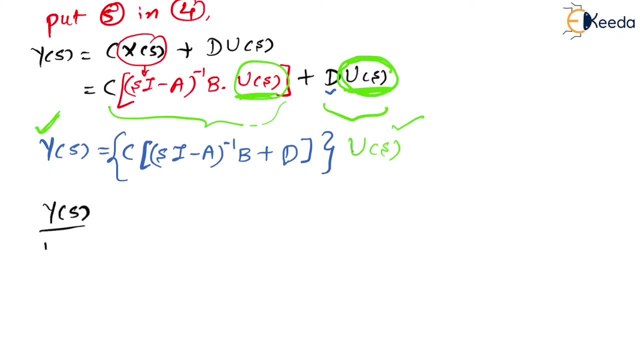 Shouldn't say that. yes, sir, What you do is you just take y of s upon u of s, You just take this, u of s, this side, and whatever you have here is nothing but the transfer function, which is nothing but equal to. yes. it is going to be c into si minus a, inverse into b plus d. 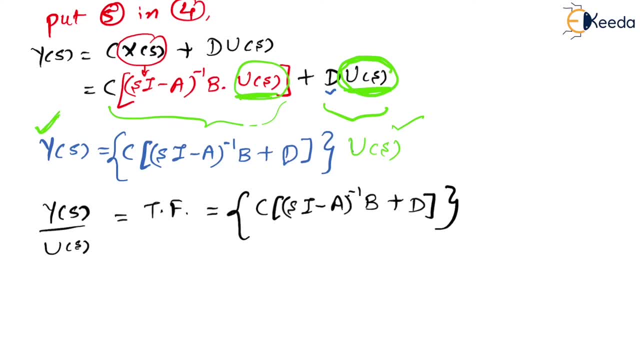 So you please do this, sir, and it is done. So this is our transfer function, if you just think of. But now my question is: Can you do this y of s upon u of s? No, you cannot do y of s upon u of s. 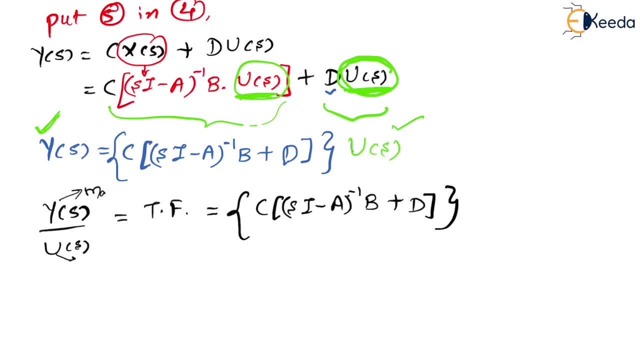 Why? Because y is a matrix, u is a matrix. This is also a matrix. This is also a matrix, And I have already told you that matrix division is not possible. So if matrix division is not possible, then this cannot be done. 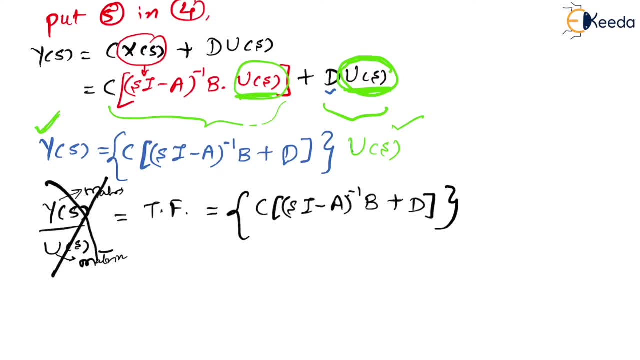 So if this cannot be done, which means I should not write it this way- I should only keep that transfer function is going to be this, only That's it. I should not write y of s upon u of s. This is the biggest conceptual mistake people do. 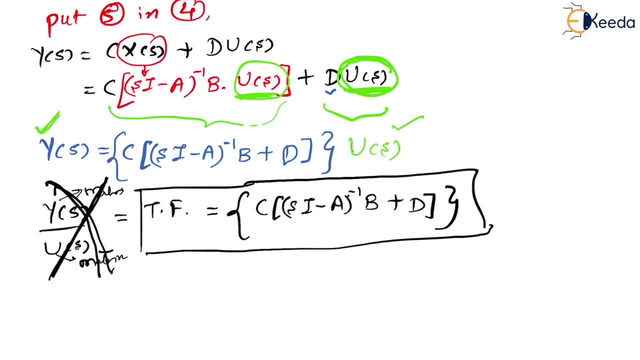 Why? Because students don't know basic mathematics, But here we need to understand everything in detail. That is the reason I have told you that, yes, saying that y of s upon u of s for the state-space model is not going to be helpful. 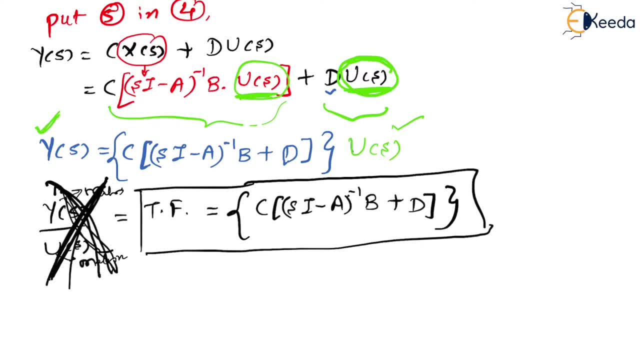 This cannot be done, So this is a clear mistake. This is very, very wrong, Right? So only our transfer function, Let me call this transfer function. T of s is nothing but going to be c into s, i minus a, inverse into b plus d. 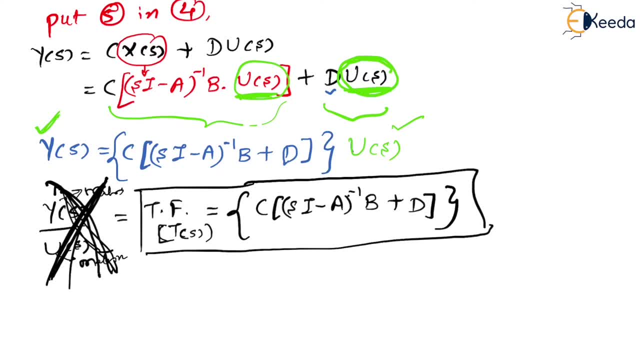 Now, the best part about this is: see here. So this is nothing but transfer: function of state-space model, of a given state-space model, Transformation of a given state-space model. Now see here. Let us talk about this term first. 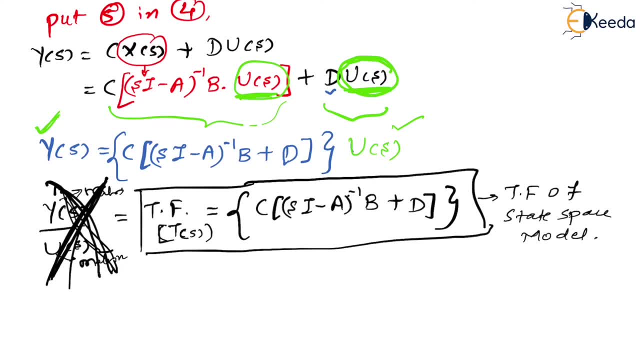 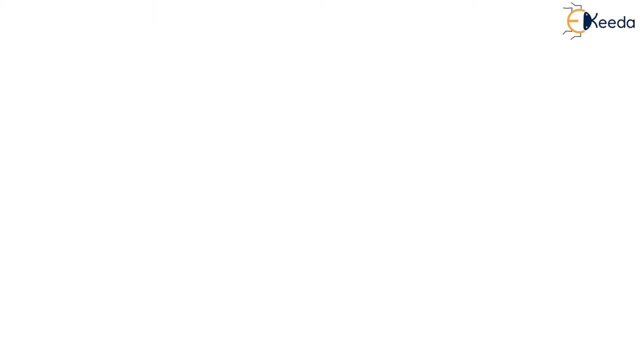 Let us talk about this And let us try to appreciate this equation. Let us try to appreciate this equation. Let me write it down again on a separate page: T of s equal to Right. This is what was the transfer function: Right. 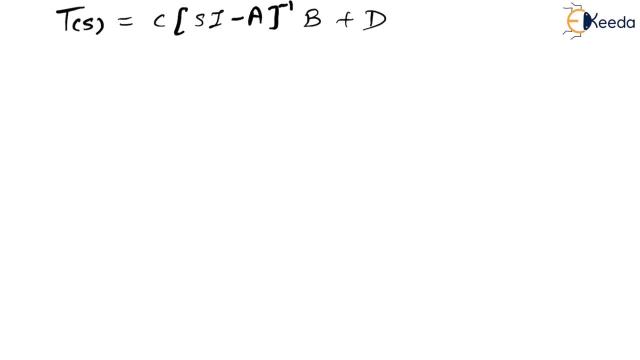 Now, yes, this is the transfer function, Right, Let us try to understand it in detail: See here, See here. So let us come on one side. Yes, We know that. if, for example, I have matrix A and I need to find inverse, 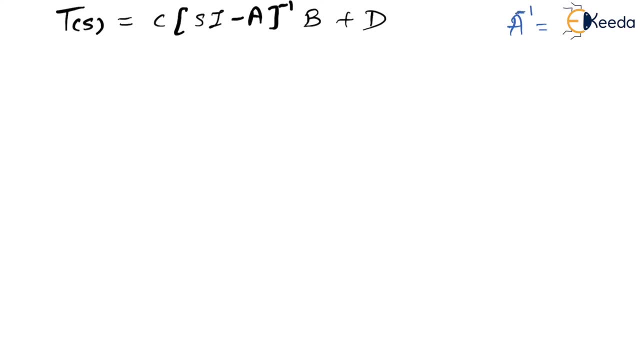 Then if I need to find inverse, what does that mean here? Which means you need to find adjoint of this matrix A and you need to divide it by the determinant of matrix A. Am I right? Yes, Because A inverse is nothing but adjoint of A upon determinant of A. 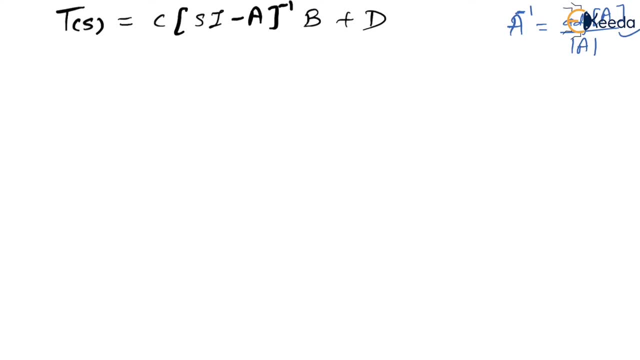 That is what we have learnt in our school days. This is what We have learnt Right. So now let us try to appreciate this equation a bit. So if you just see here by the same logic, if you see this equation, can it be written in the same terms? 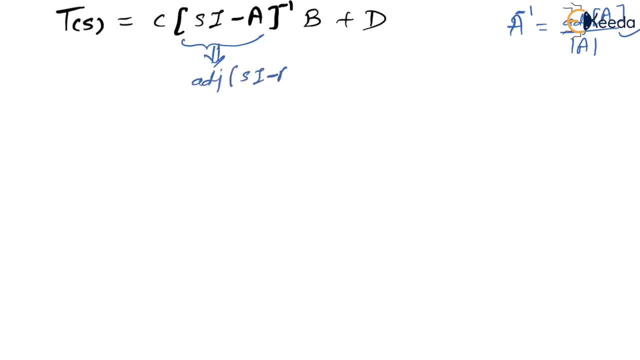 Means. can I write it as adjoint of S i minus A upon determinant of S i minus A? Can I write it? Yes, definitely. So let me just write it this way and keep the other things same. So this is T of S, which is equal to C, into adjoint of S, into B plus D. 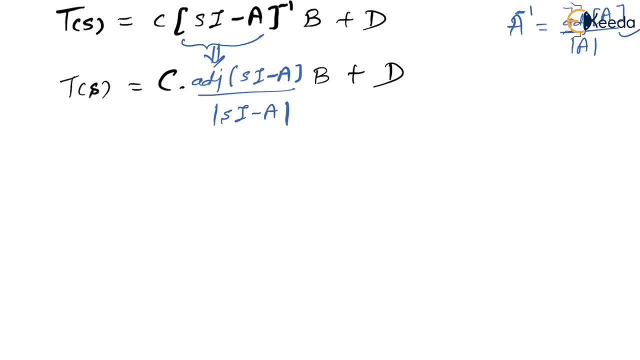 Is it alright? Yes, Because S i minus A inverse can be written as adjoint of S i minus A, divided by determinant of S i minus A. That is what we know. Now let me consider a MISO system such that you will understand what I want to say. 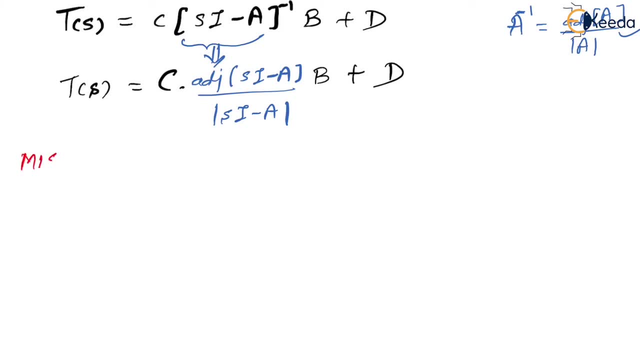 Let me consider a MISO system. Let me consider a MISO system. Okay, Yes, Now MISO system in the sense multiple inputs and single output. Right, Multiple inputs and single output. So output is just going to be same. 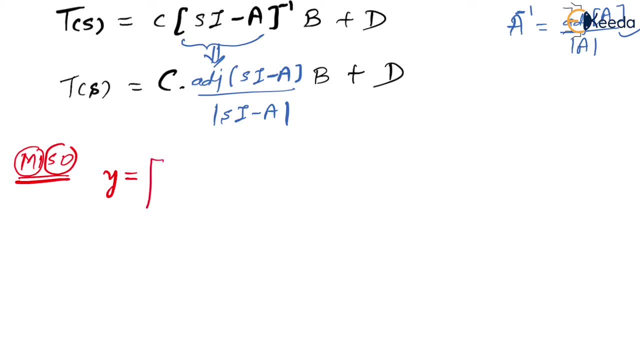 So let me consider: yes, output is 1.. So let me consider 1 output And I will be having this particular transfer function like sort of right Right here. So this is basically, if I think of this is not small. 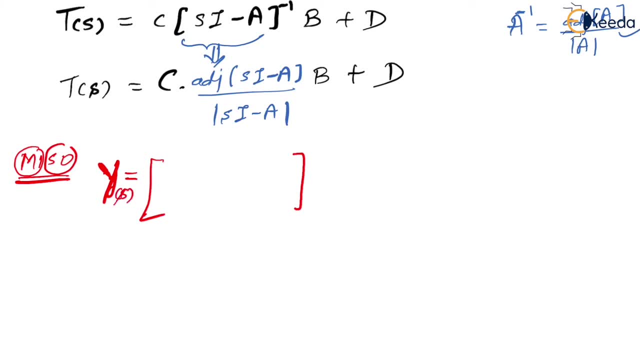 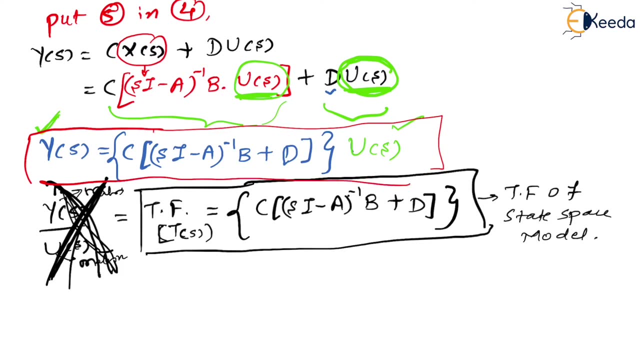 Let me think of this in Laplace domain. only Y of S. See here. Let me consider this way, only this equation. Let me consider it in this equation, formally Right. So yes, definitely, this Y of S is a matrix. 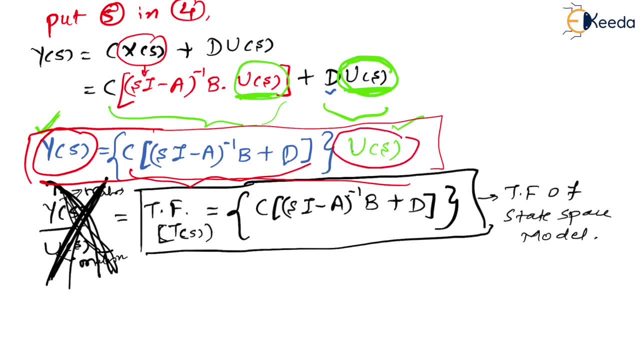 And this everything is a matrix, And this U of S is also a matrix. So, yes, U of S. yes, Now it is going to be multiple, So let me consider 2. U1 and U2 inputs. 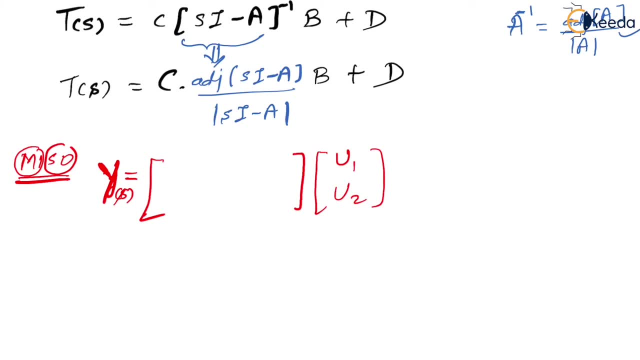 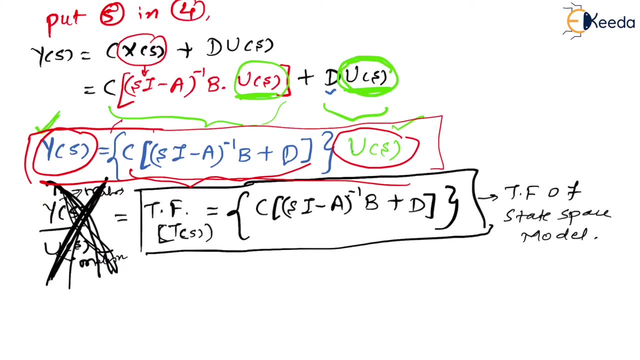 Is that right? Let me just consider 2 inputs for now. So it is definitely going to be MISO system right Now. yes, Do you agree with me that whatever is there in this blue, whatever is there in this blue, return this same thing? 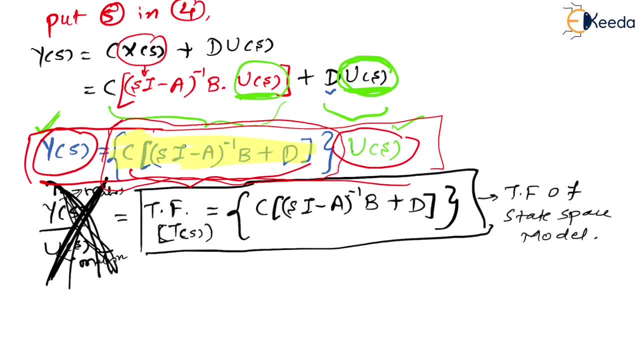 this whole thing. if you see this one, this whole thing: C into S, I minus I inverse into B plus D, right, If you think of this whole thing, this whole thing is just simply matrix, or not? Yes, it is going to be a matrix. 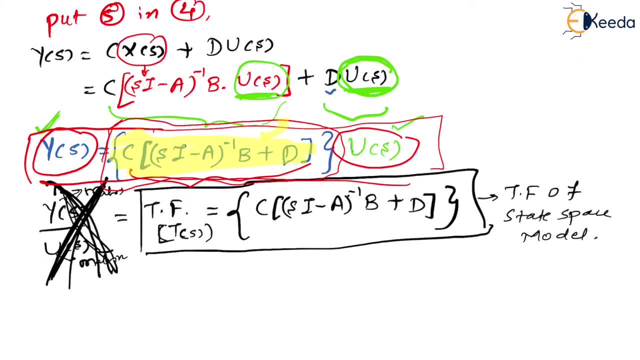 So, and if you see here it is going to have things in S, It is going to have things in B domain only. Yes, definitely, because C will have some of the other stuff and this is just going to be that way. 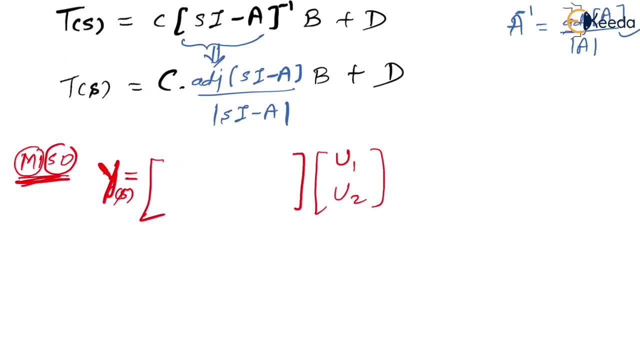 So let me just consider those transfer functions. So yes, Inside this I may have let us say S1 upon S1 plus S2.. Or I may have let us say S3 upon S4 plus S5.. 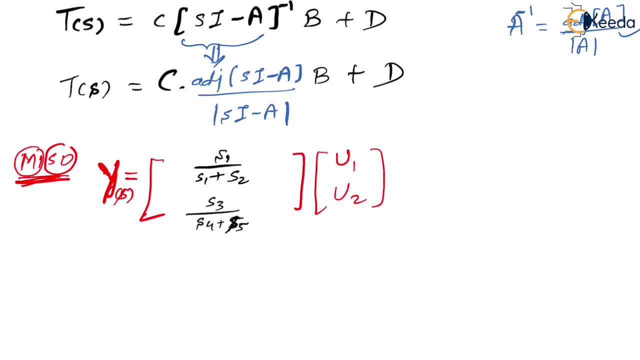 S5. S4 plus S5. I may have such kind of transfer functions, Right? So if I am having such transfer function, if you just think of this Y by U1. If you think of Y by U1, then, yes, definitely Y by U1 is going to be S1 upon S1 plus S2.. 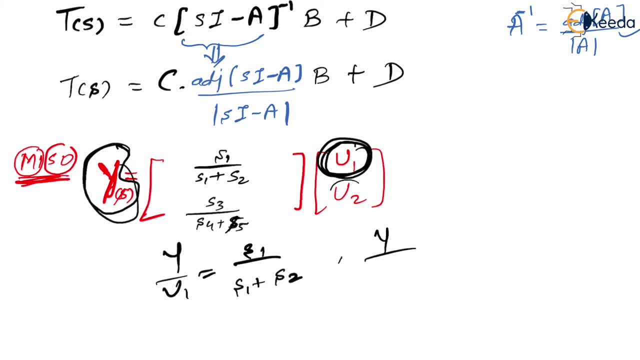 Similarly, if you think of this Y upon this U2, this U2.. So, yes, definitely it is going to be S3 by S4 plus S5.. Now, what do you understand from here? What do you understand from this one? 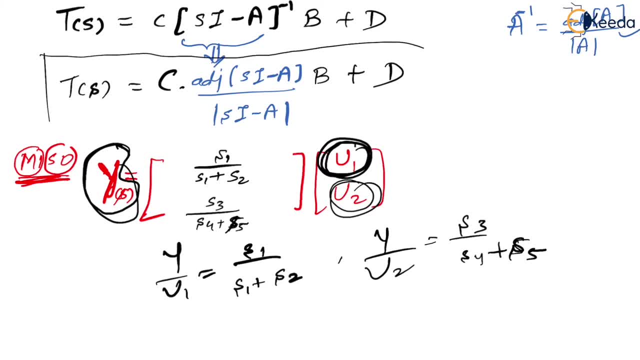 You understand that after computing this T of S, it is not necessary that you get a single transfer function. Rather, you get a single transfer function only for SISO system. But since it is a MISO system, you are not going to have a single transfer function. 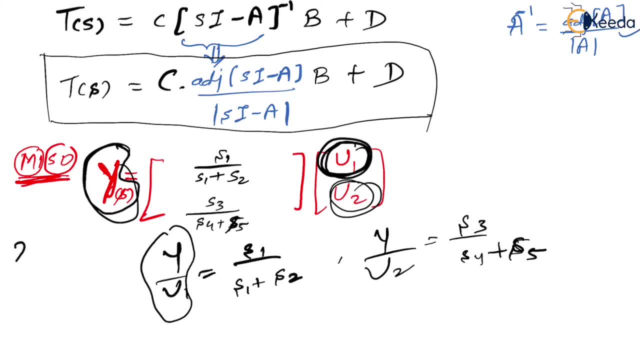 You will get two transfer functions here, because it is MISO, Because it is two input And one output system, Right? So here you have got just two transfer functions. So this, yes, you may see that while looking that, yes, this is only one single equation. 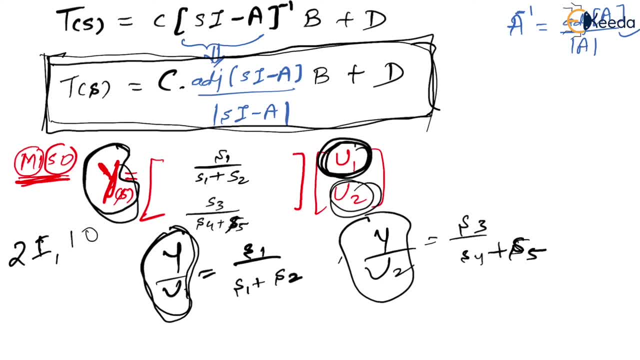 Yes, this transfer function is a one single equation, only One single. what do we say? one single matrix only, But, but. but it is a one single matrix only, But you can compute. yes, definitely, you can compute one single matrix only. 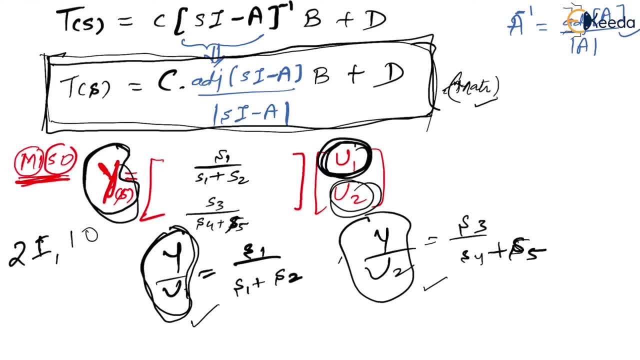 Definitely, you can compute more than one. More than one. what do you say? transfer functions out of it, Right? So this is the first thing you need to note. Other thing is: let us think of a SIMO system. 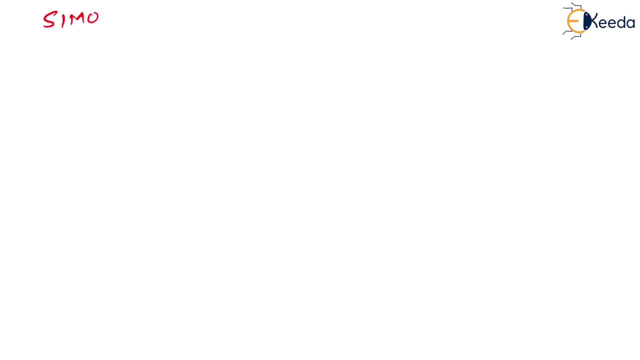 Let us think of a SIMO system. If I think of SIMO system, what does that mean? That means that output is just going to be one. So let me call it as U And yes, definitely yes, It is multiple outputs. 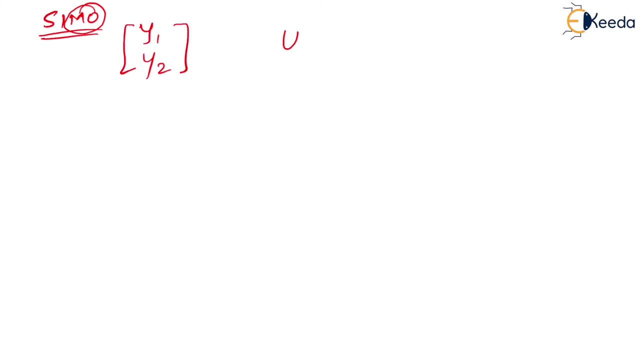 So multiple outputs means- let me consider this- Y1 of S and Y2 of S, Okay, And in between I am going to have some matrix Right. So even here, if you see, you are going to get two transfer functions. 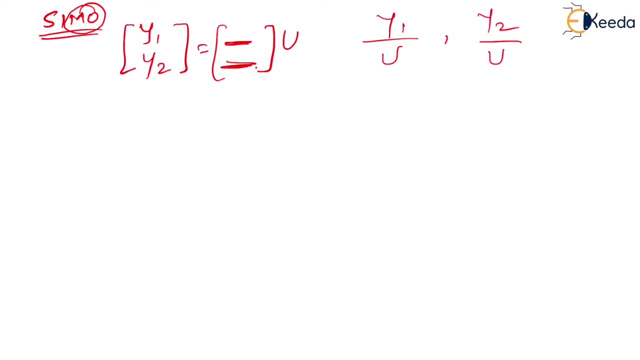 That is Y1 by U and you are going to get Y2 by U, Right, Yes? Now let me consider MIMO system. If I consider MIMO system, MIMO system means let me consider two inputs And two outputs. 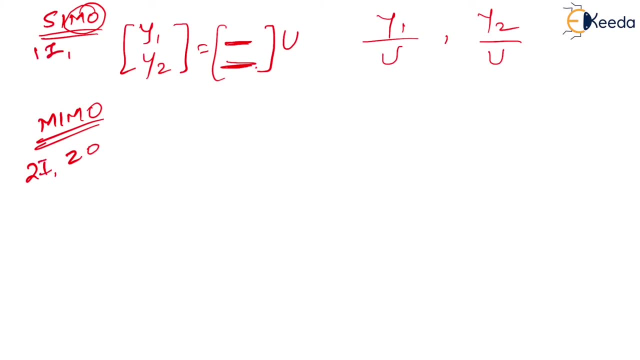 Right Here, I was considering one input and I was considering two outputs, Right This way. So now let me consider here also, Let me consider two outputs. The moment I consider two outputs, it is going to be: let me consider Y1, Y2.. 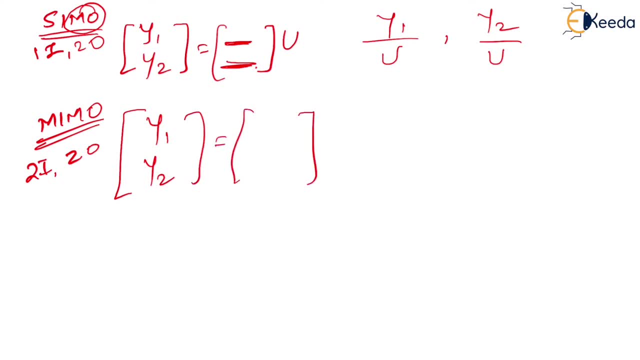 And yes, definitely, there is going to be some matrix here And you are going to have this U1 and U2.. Right, Yes, Now, definitely we know that this matrix in between, which is there, is nothing but a. 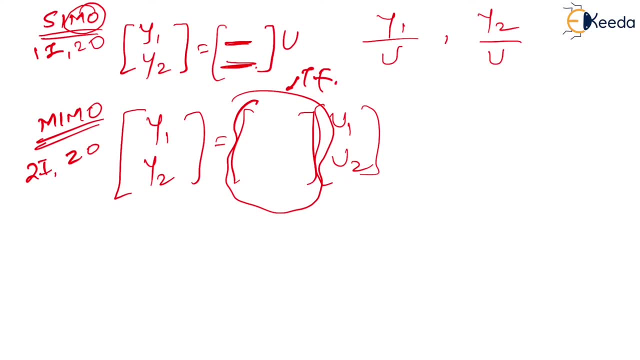 transfer function matrix only. We have already seen. But if you just think of this one transfer function matrix has so many other transfer functions also, Means this transfer function matrix will also give you Y1 by U1.. It will also give you Y1 by U2.. 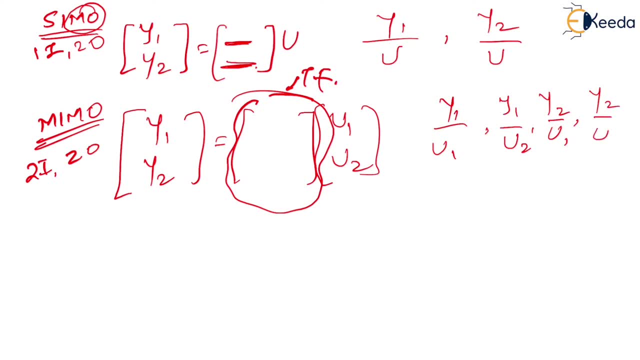 It will also give you Y2 by U1.. And it will give you Y2 by U2 as well. So here it is going to give you four transfer functions. Here it is going to give you two transfer functions. 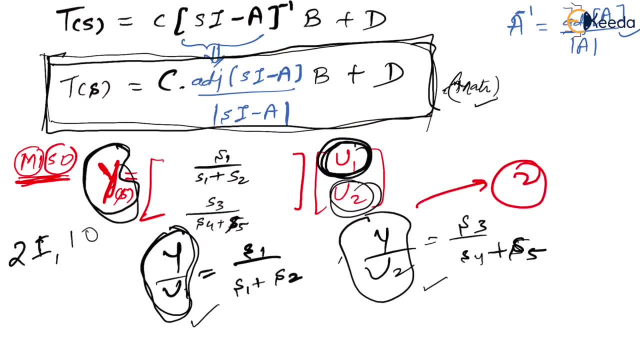 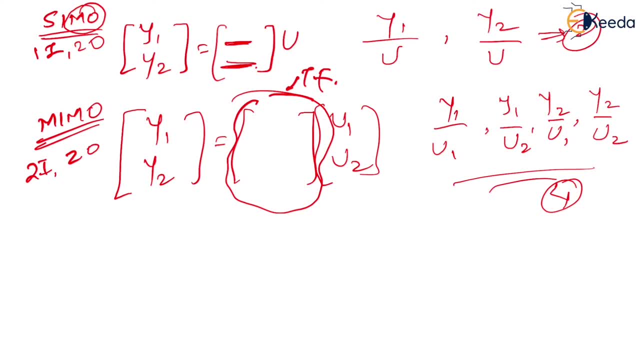 And in the previous case also, it is going to give you two transfer functions. Now, what is the more known? What is the moral of the story? Moral of the story is that the total number of transfer functions present in the T of 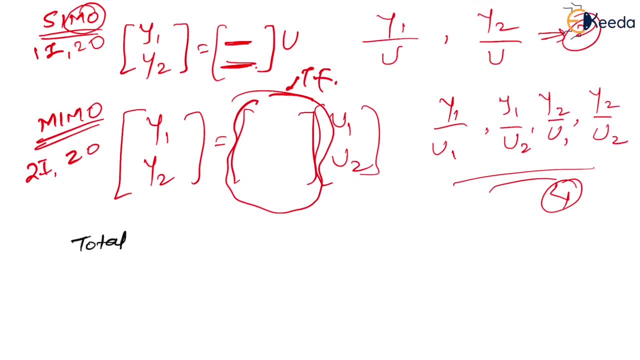 S. Let me just write it down. Total number of transfer functions in T of S. See, T of S is going to be one single only, But that one single itself is having so many other transfer functions also. How do you understand that? 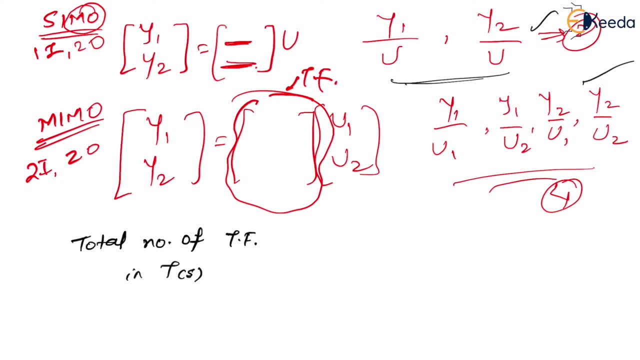 You just understood that by these examples, Right? Anyways, So if you just see here, So after computing T of S from the state space model in T of S, After Right, So the total number of transfer function in T of S is going to be number of inputs. 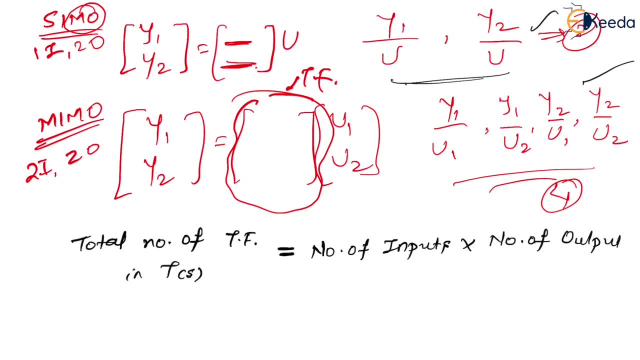 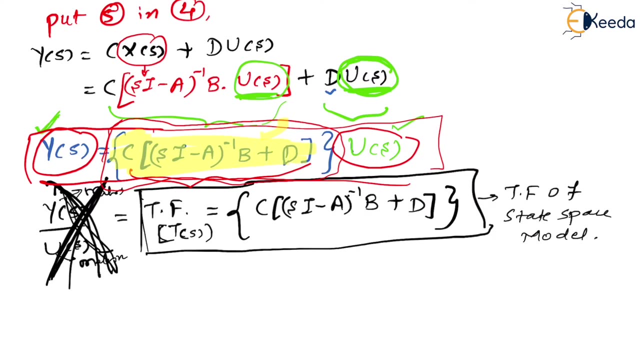 multiplied by number of outputs. This is very, very important. Let me just revise it very quickly, Very quickly See, Basically, we just saw that, yes, this was the transfer function. we understood Right Now, yes, When we understood that it is a transfer function. 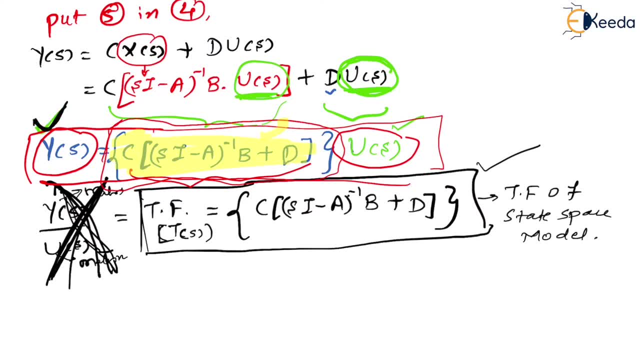 So we just tried to apply this here to this particular equation: That Y of S equal to C into SI minus A inverse into B plus D into U of S. So what we tried to do it, Yes, We just tried to replace this C into SI minus A inverse into B plus D as T of S. 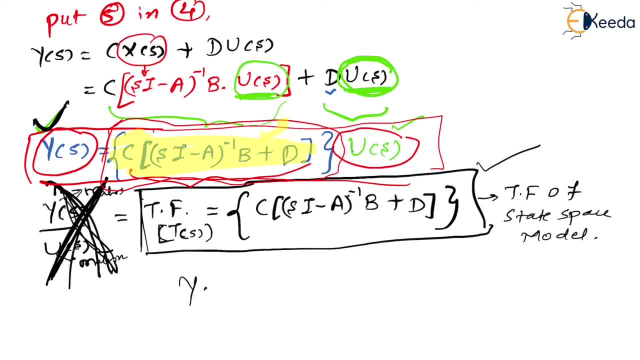 Right, And we just tried to show the terms in terms of Y of S, equal to, let us say, T of S into U of S. In such terms We tried to show it Right. So even there, if you see, If you just show this, 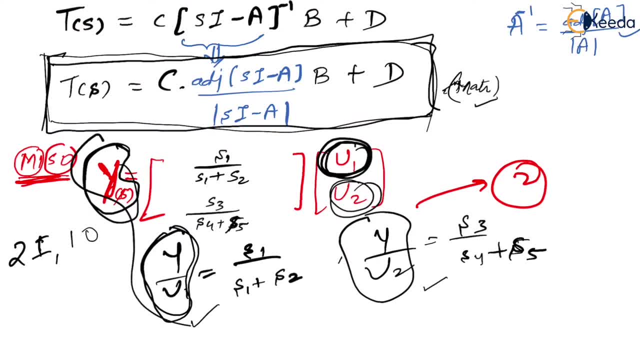 Means in this particular fashion. We have shown all of this Right, We have shown all of this. So when you show it this way, you understand that the center one, The center one, The center one here, This blue is going to be the transfer function. 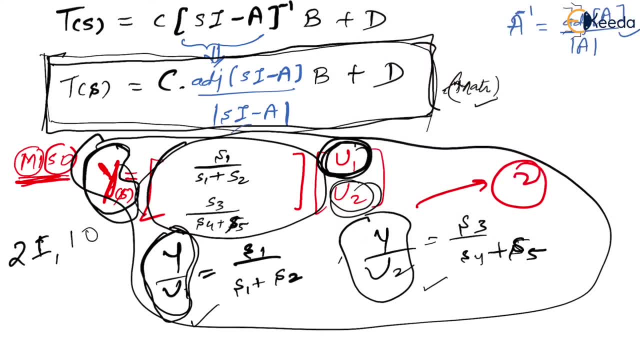 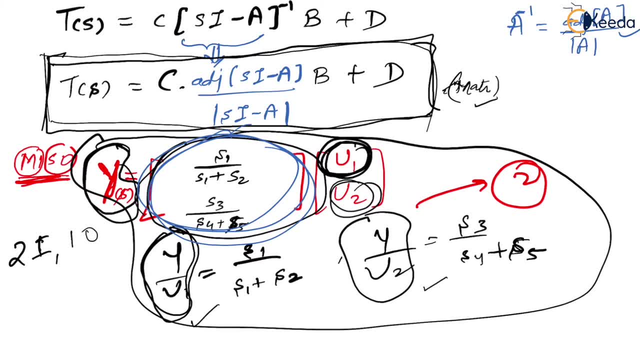 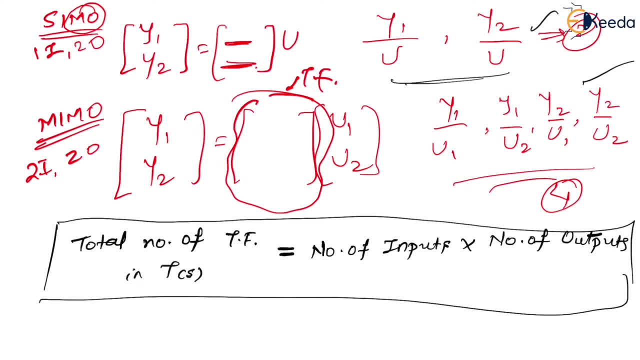 having some modular transfer function. But yes, Definitely by this. if you just compute the equations, The equations if you think of, Then you get Y of S upon U of S and Y of S upon U of S as well. Similarly, here also, you get Y1 of S upon U of S and you get Y2 of S upon U of S as well. 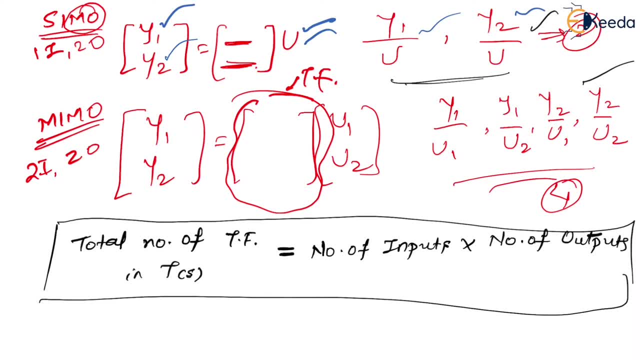 So these are two equations that you get. You get the two transfer functions, Means within the one single transfer function, Within one single transfer function that you have got from the state space model, now going to have so many other different transfer functions and the number of those transfer. 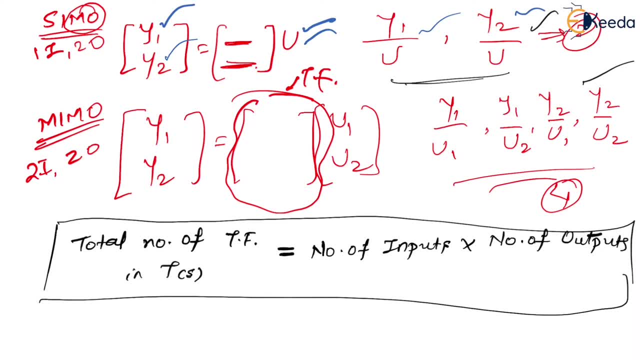 functions which will be there. present in that one single function which you got from the state space model is going to be number of inputs into number of outputs. you may check this. if you just think of this, see what is this. this is going to be one input and two outputs, so it is going to be one. 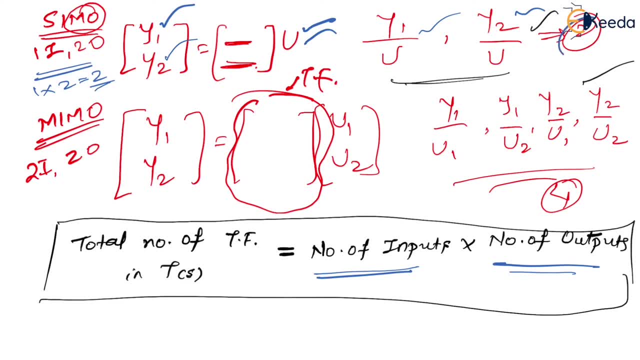 into two, which is two. are there two transfer functions or not? yes, definitely here, two transfer functions we have got. similarly, if you see, here you have got two inputs and here you have got two outputs, so it is going to be two into two, which is going to be four. so do you have here four? yes, 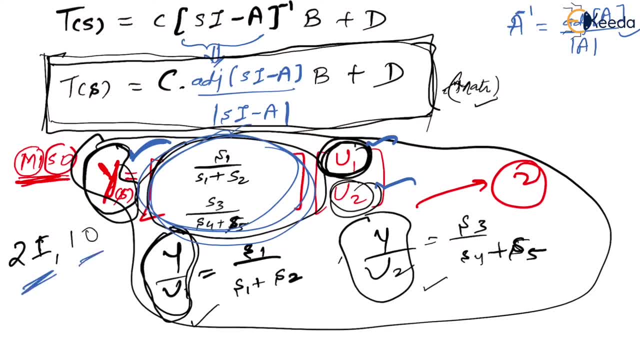 definitely you have here four. similarly, if you think of: yes, this has two input and this has one output, it is two into one. so number of inputs is two, number of outputs is one. so multiply them, so two into one is going to be. yes, is going to be two. so do you have here two? yes, definitely you have. 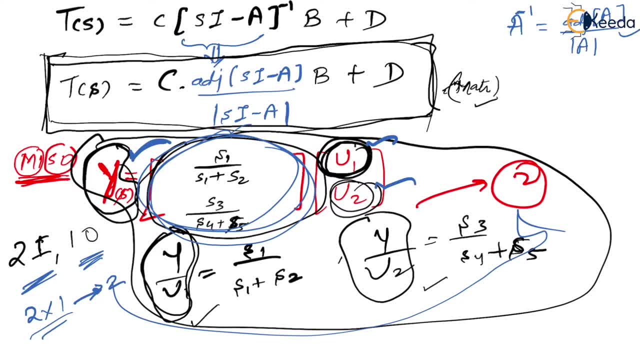 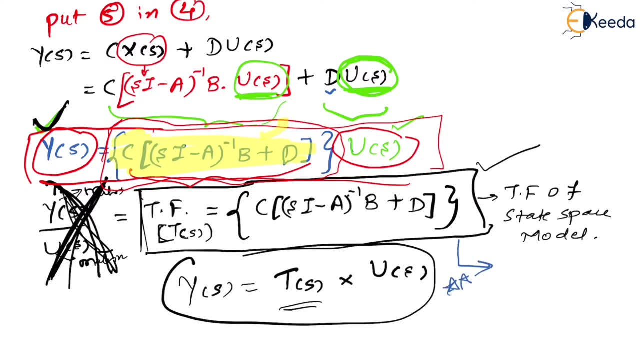 this is the way we have now. the most important point, most important point out of all of this is: see, most important point is: whatever transfer function you have got here right, whatever transfer function you want- this is very important point- keep it. two star, three star, how much star you want? please keep it, this particular. 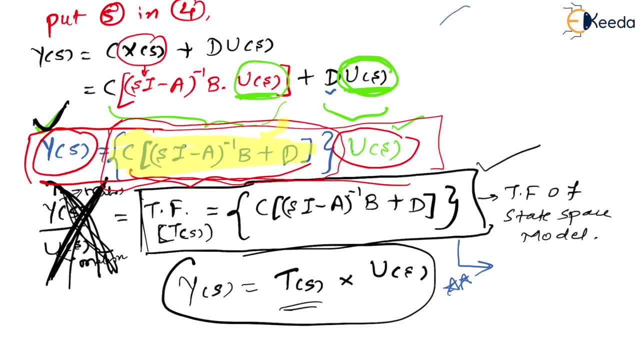 transfer function. if you just see, yes, in general, how many types of transformation we have loop gain, or we also say it as open or transfer function, and you also have closed loop transfer function, right, overall closed loop transfer function. so this particular one, this particular transfer function which is there, which you have got from the state space equation, is nothing but. 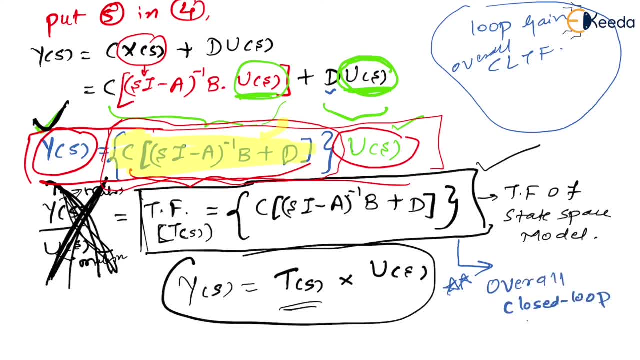 overall closed loop transfer function. this is very, very important and please remember this point. it is going to help you in exam very much because what happens is many of the times they may ask you questions related to errors in others. if you see we have those right, we have kp equal to limited extension 0 and all stuff like that, so that we apply for. 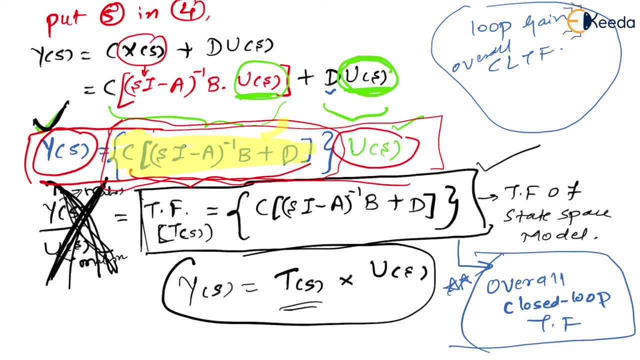 open loop transfer function, or we can say for loop gains. but here, whatever you get here from this, from the state space model, whatever transfer function you have got is overall closed loop transfer function. so you need to convert this one to firstly open loop transfer function and then apply those. 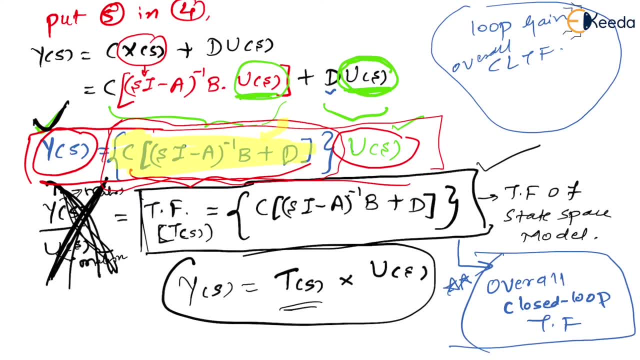 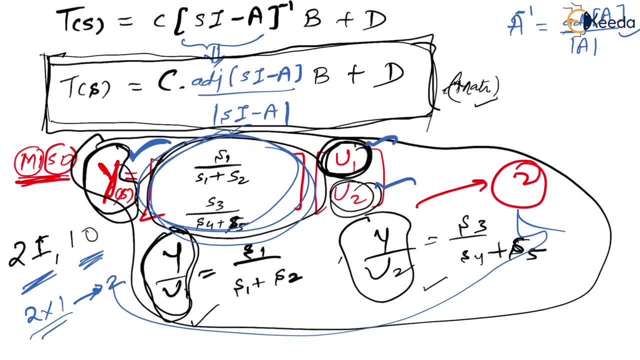 error stuff. right, anyways, let us think of next one now. yes, another observation that we need to have is: see here, see here this one, come on, very important: focus on this equation, focus on this equation. if you just see here, i will tell you that why a is called as a system matrix, why a is called as a system matrix. if you, 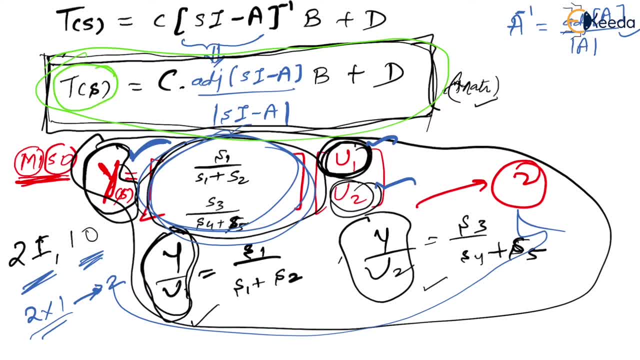 just say here: do you agree with me that it is a transfer function? yes. do you agree with me that it is the overall closed loop transfer function? yes. so what does the denominator of a transfer function suggest? denominator of a transfer function suggests that it is going to be. 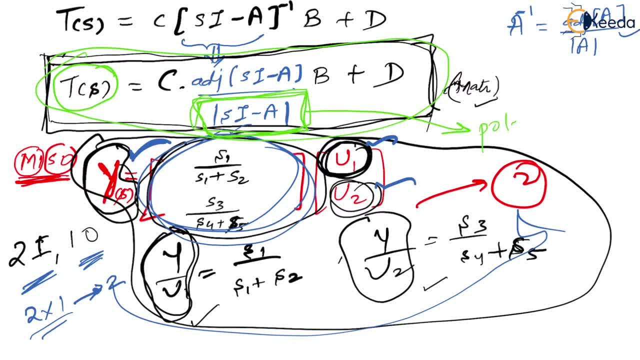 poles of the transfer function. so these are nothing but poles. basically determinant of si minus a is going to give you poles, am i right? and what do poles define? poles define stability of the system or not? yes, definitely, because whatever is the input or output, you do not consider see if your input is unbounded, definitely, output is going to be. 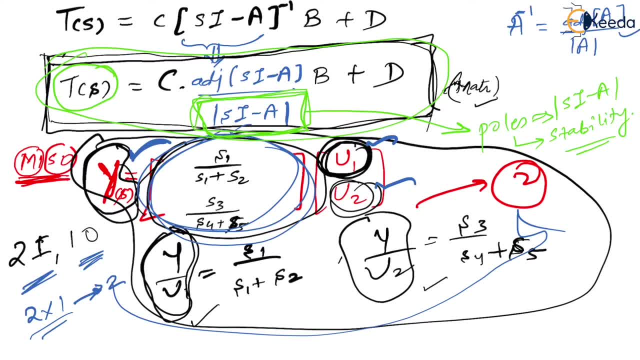 unbounded, only right. so you don't think about inputs and output, irrespective of inputs and output, if you just need to check whether the system is stable or not. so for that you just have only one method, that is poles. so the poles, if you see the poles here, if you see si minus a, si minus a. 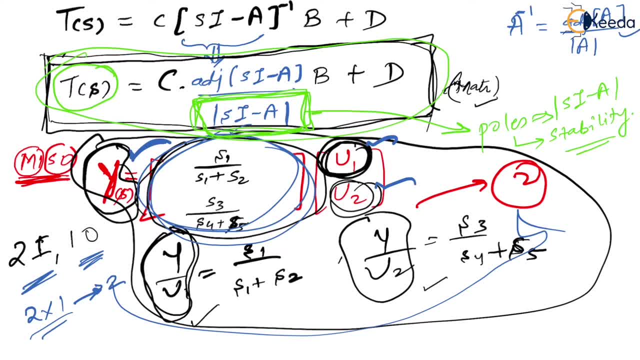 to be specific, determinant of si minus a, will give you poles, will give you poles and poles define stability, right, and it defines stability of what, stability of a system. so you can put here conversation volume if you want for saying is something simple like a number, okay, it is not difficult, but that maybe has some 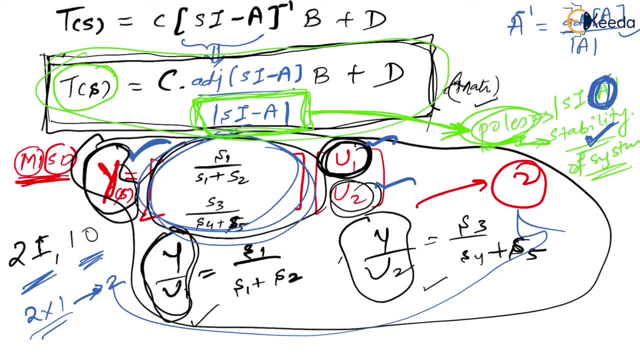 kind of complication because of some kind of surname. anything else is going to be a Tails and a value hadn't been marked before. so, which means that we have two points�, car you are going to finding a onion and thatvy. we are going to find out just one point, which is very important as it has to maintain just magical stability and the curve. now, if we think about pull this three things here, if we think of a, these, a, these, a, which is called a system matrix, it plays a very, very important role in defining stability of the system. that is the reason we call a as system matrix. i hope you are understanding this point. now let us try to take some examples related to the something, yes, the example, if i take the same. 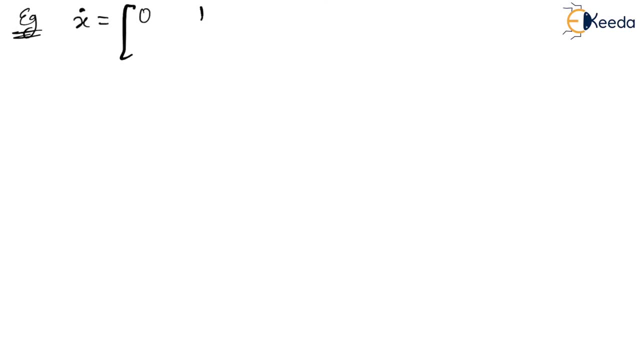 Let me consider that you have a state space model, Yes, So you need to find the transfer function for the same. Now you please tell me what is the transfer function T of S for a state space model? It is going to be what? 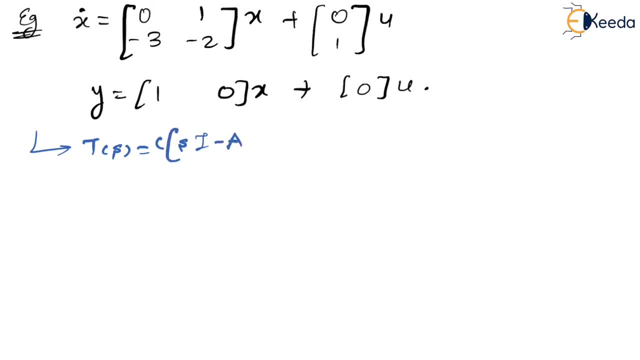 Yes, it is going to be C into S i minus A. inverse into B plus D. Am I right Now what you have got? Let me first try to find S i minus A And then I will just do the stuff. The remaining stuff. 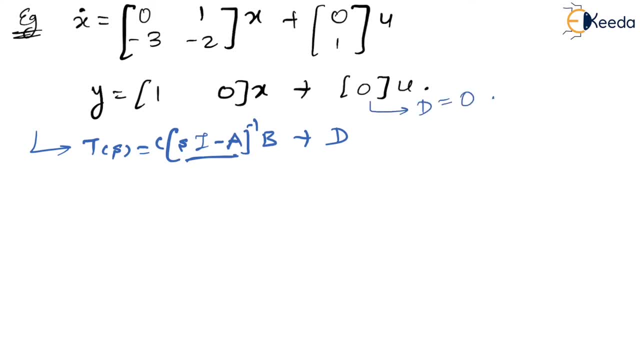 If you just see here from this equation what you get, You get that D is equal to 0. So there is no need to consider this D, It is gone. Right Now let us try to find S i minus A. first, 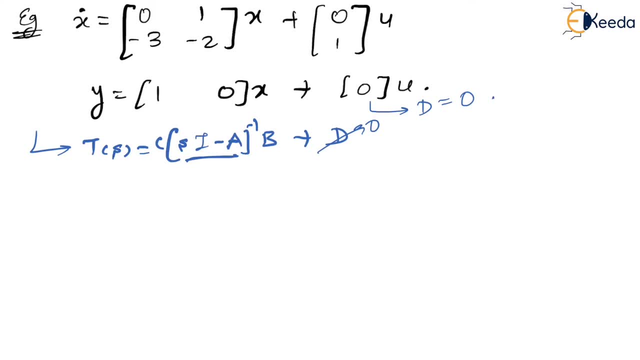 And then we will find S i minus A inverse also, And then we can do the rest of the thing. Yes, So if you just see here, Yes, How to find What is S i minus A S i, What is S i? 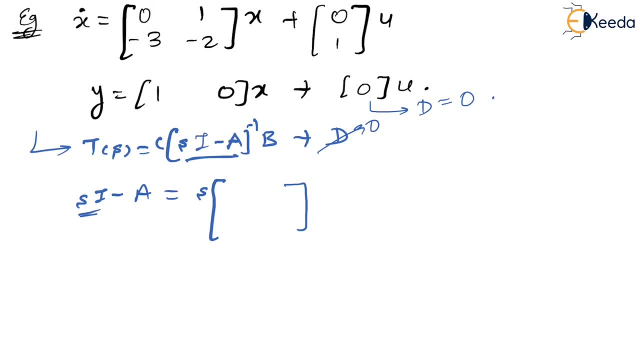 S is nothing but S into identity matrix, Right? So identity matrix is what It is going to be: 1, 0,, 0, 1.. Identity matrix is a matrix whose diagonal element Elements are 1 and of diagonal elements are 0. 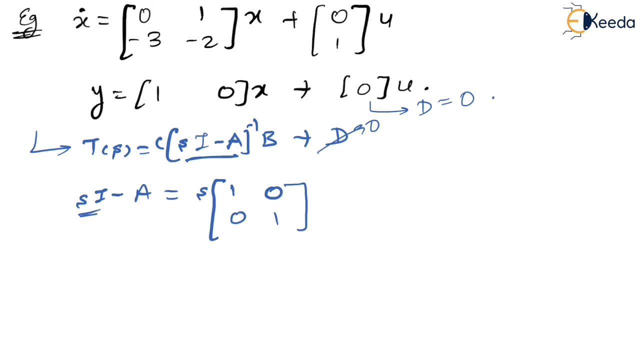 That's it. Or we can also say that identity matrix is a diagonal matrix with diagonal elements as 1.. That is a diagonal matrix, So this S into this one minus A. What is our A? Yes, A is going to be 0, 1, minus 3, minus 2.. 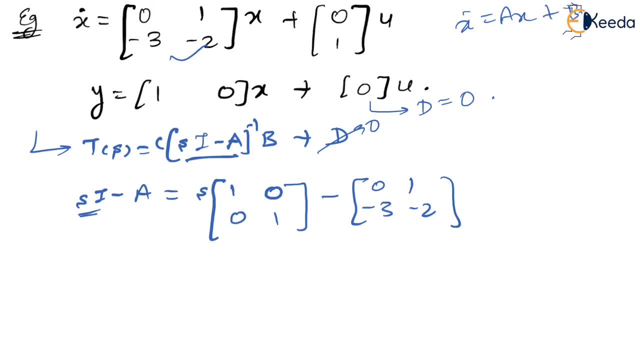 This is A Right, Because we know that X dot equal to AX plus BU. So whatever you have, Dependent on X is going to be A. So dependent on X is going to be A. So this has to be definitely. 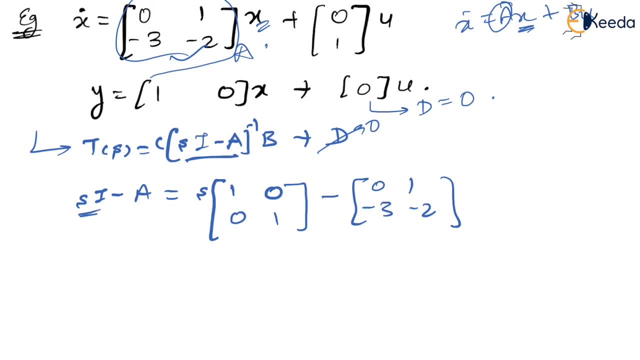 This has to be definitely A matrix Right? Yes, So this is the way we have done. So let me just do it. Let me just simplify it further. So this becomes S 0. This S multiply, Multiply everywhere. 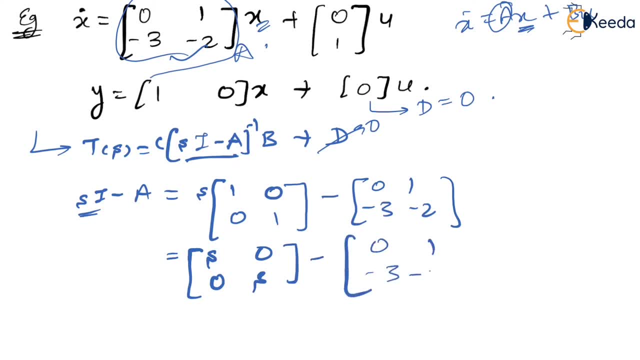 So this becomes 0. S Minus, If you think of 0, 1, minus 3, minus 2.. Now you just add them linearly, So this becomes S i minus A If I just add them. 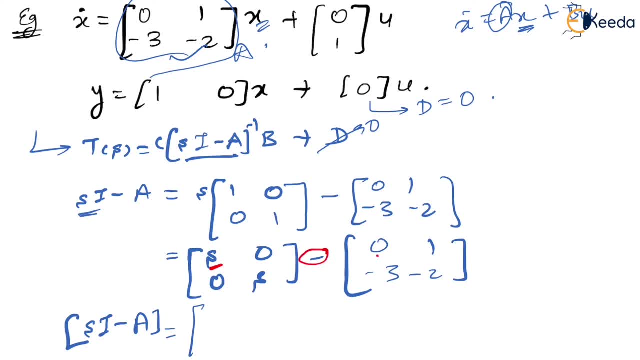 If I just add them, What do I get this? This S minus 0 is going to be S. Similarly, 0 minus 1 is going to be minus 1.. Similarly, this 0 minus of minus 3 is going to be how much? 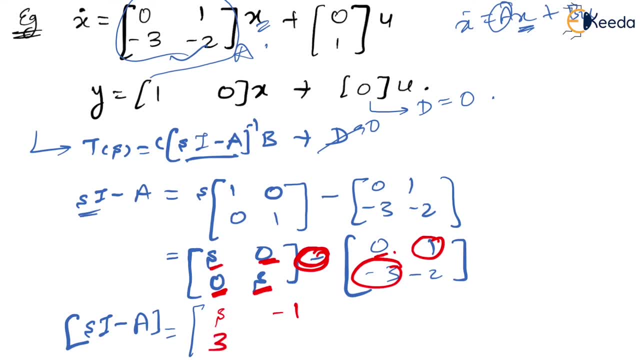 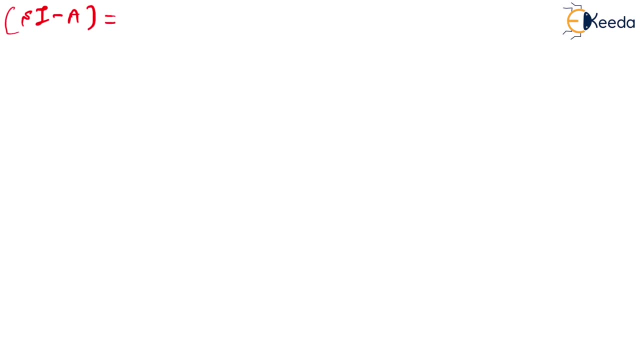 0 minus of minus is going to be 3.. Then, yes, S minus minus 2 is going to be S plus 2.. So this is S i minus A. So I have got that. S i minus A is going to be what. 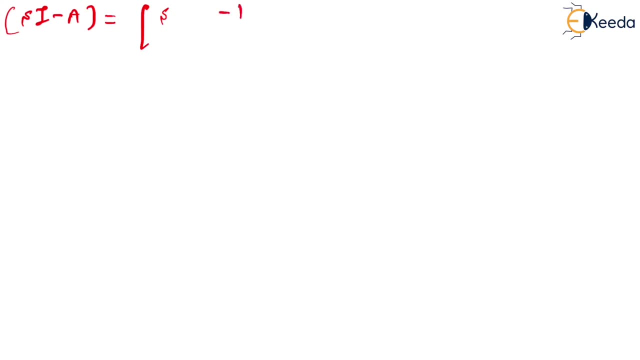 Yes, It is going to be S minus 1, 3, S plus 2.. Now the point is what we need to find. We need to find its inverse. So for 2 by 2 matrix, let us come aside. 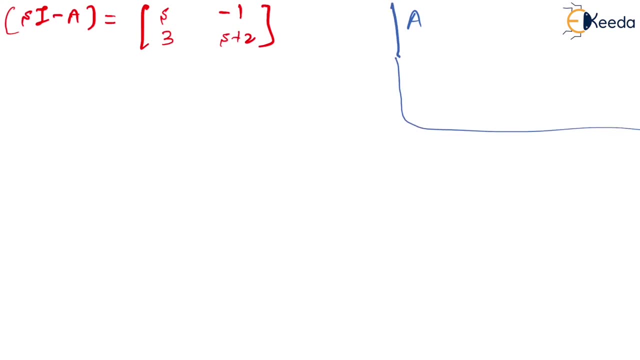 Yes, If, for example, you have, let us say: this is, for example, only right. This is, for example, If you have A right A matrix having element, let us say A, B, C, D. 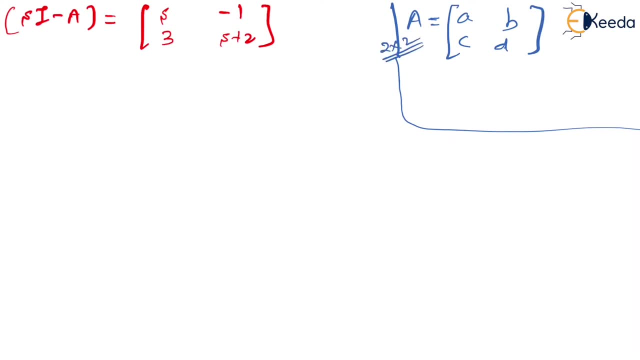 If it is a 2 by 2, this it is a shortcut. It is a shortcut for 2 by 2 matrix only. By the way, let me just tell you: Yes, So this S? i minus A. If I need to find inverse of this, this becomes S? i minus A inverse. 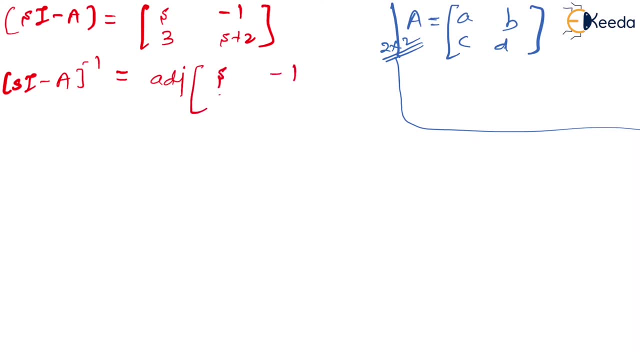 which is nothing but what Yes Adjoint of this S, S, i minus A, divided by determinant of S, 3, minus 1, S plus 2.. Right, Divided by the determinant. Now, what do you need to find? 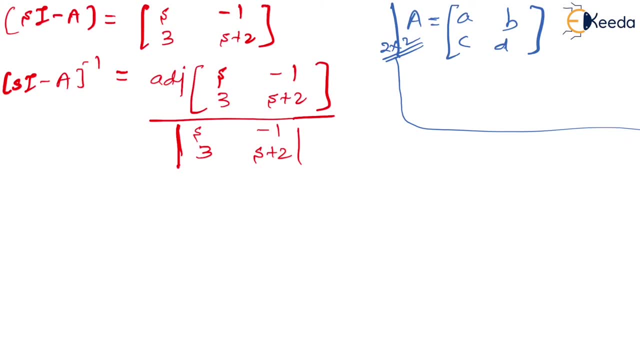 Yes, There is a shortcut, because in order to find adjoint, there are so many steps. You know, do you first find minors, then, after finding minors, you please find cofactors, And then you know stuff like that people do. 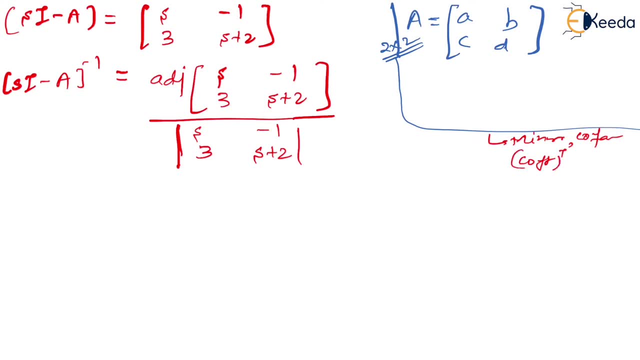 And then you know, yes, cofactor matrix, whatever you have got transpose of that cofactor matrix will give you adjoint right. This is what is the rule which right Now, But we need to apply Shortcuts in gate. 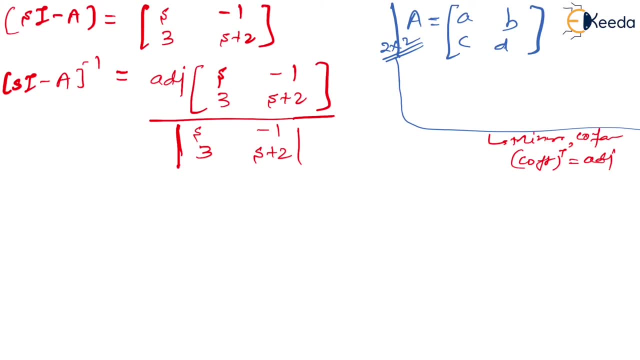 So what is the shortcut? to find adjoint, See, determinant can be easily found out. No, such this thing. Hurry in it, right, But problem is with adjoint. So in order to, because who will find minors, cofactors and then take the transpose of that matrix and all? 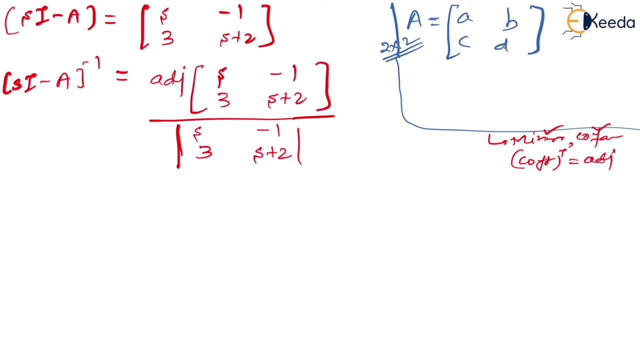 We don't have that much time in gate, So for that we have a shortcut. What is that shortcut? Shortcut says that whatever diagonal element- let me consider this adjoint of A. Okay, Yes, Let me draw this adjoint of A. 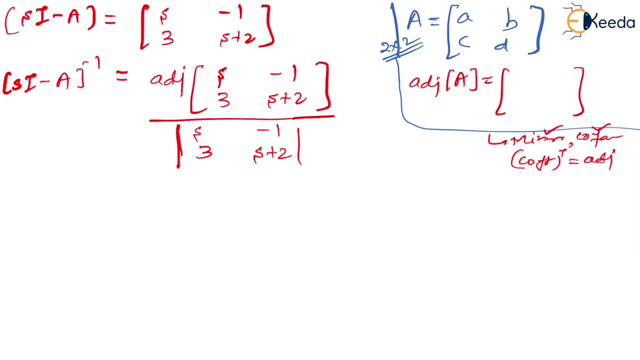 So, yes, What does that say? Whatever diagonal elements you have, you please flip them. Whatever diagonal elements you have, you please flip them. So, you please flip them. So let me have this D here. Let me, because this D will now go in place of A and this A will now go in place of D. 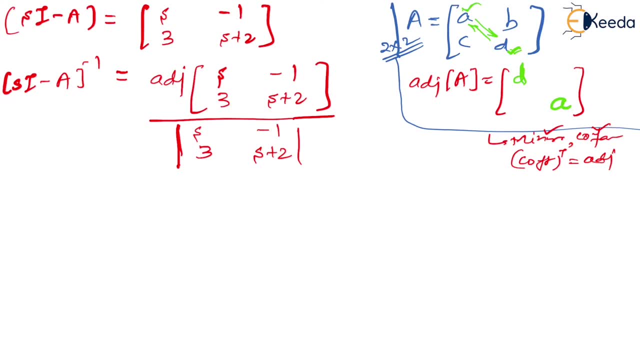 So here comes A, Is it correct? Yes, Slowly, slowly, slowly, No need to worry. Yes, And what about other elements, All diagonal elements, that is, this B and this C. you please change their signs in their respective position only. 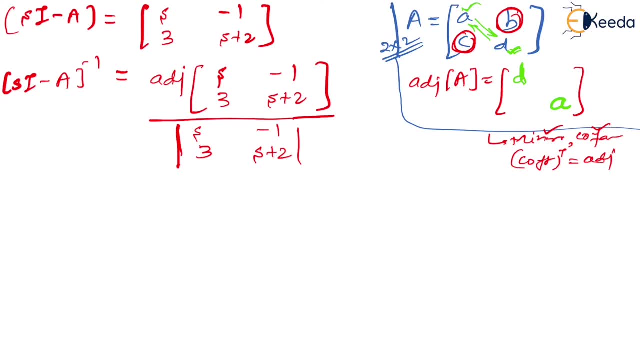 Means you don't need to flip B and C. You please change their sign at their place. So, minus B, minus C. This is what is the shortcut. So you please apply the shortcut here and you get that. Yes, you need to flip this too. 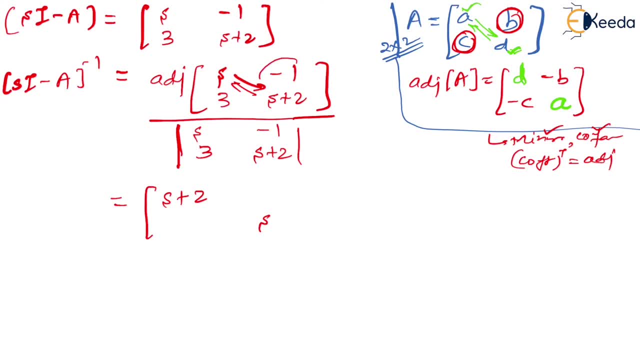 So just flip this too. You get S plus two and you get this S, and you just need to change their sign. So this is minus one, So sign is going to become plus one. This is going to be plus three. 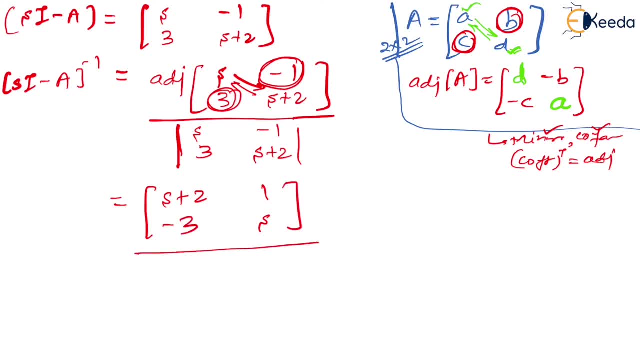 So sign is going to become minus three. This is the adjoint, And now here at down, you need to have the determinant. So, to find determinant, what do you do? Yes, This into this, minus, this into this. So you just do that. 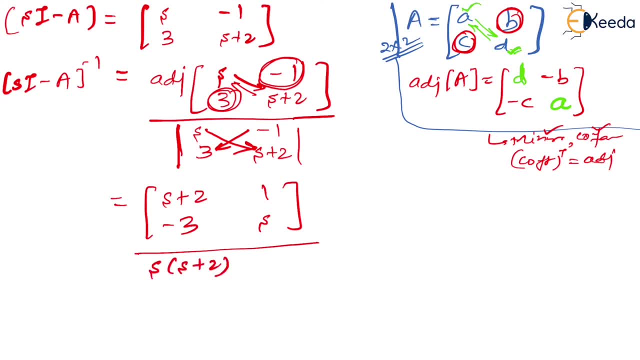 So this into this is going to be what Yes, S into S plus two, And this is going to be minus, minus of three into minus one. Three into minus one is going to be minus three. Am I right? Yes, definitely. 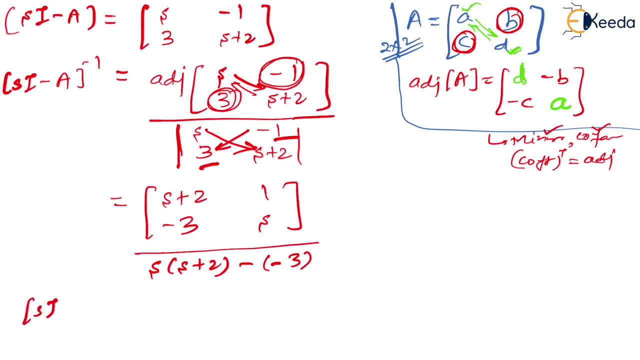 So, from this, what you get is: yes, you get that S I minus A inverse, S I minus A inverse is going to be what One upon, if you think of this is S into S is going to be S squared plus S into two is going to be two: S plus three. 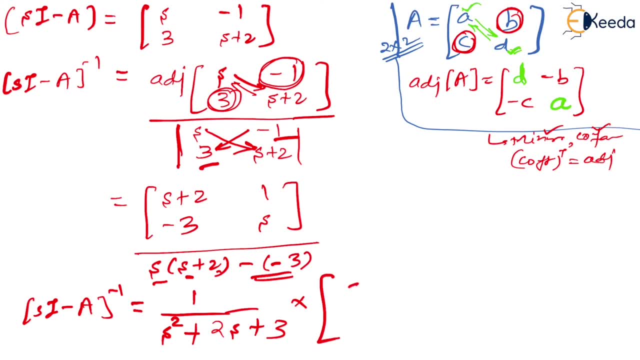 This is going to be plus three, This whole thing multiplied by S plus three. So this is going to be minus two, one minus three and S. Is it all right? Yes, definitely. Now do we need to stop here? 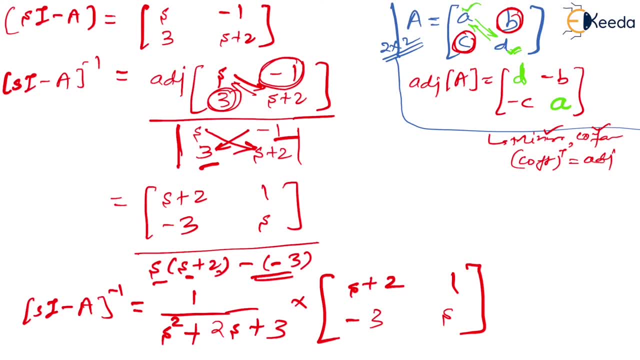 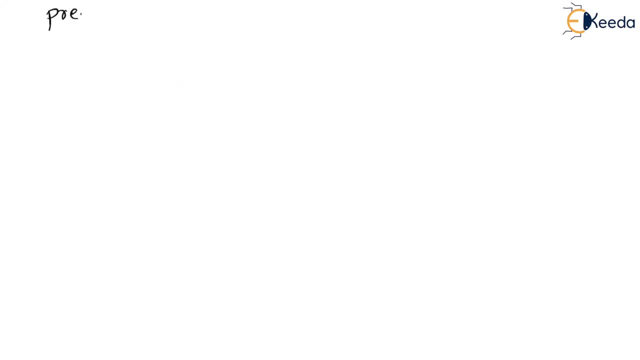 No, because we need to find C into S, I minus A inverse into B, right. So let us pre-multiply by C. Let us pre-multiply by C and see what happens. So the next step: Pre-multiply by C. 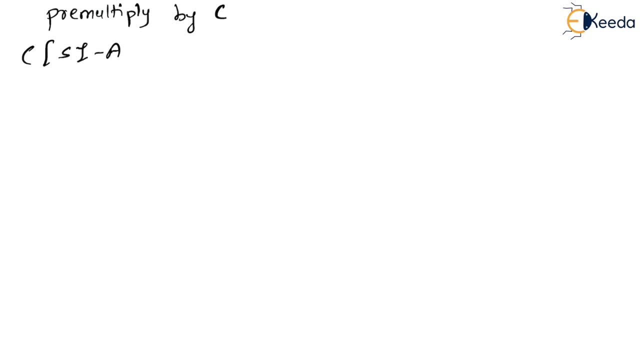 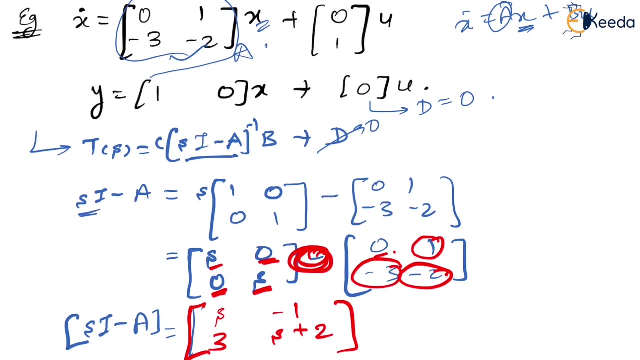 So this becomes C into S I minus S. I minus A. inverse right: S I minus A. only It is going to be yes. What is C matrix here? Yes, this is going to be C matrix. C is going to be one zero right. 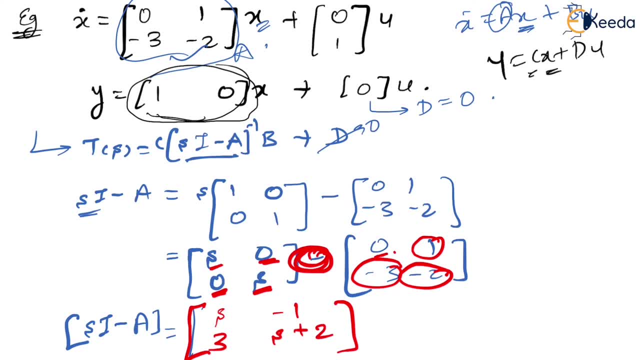 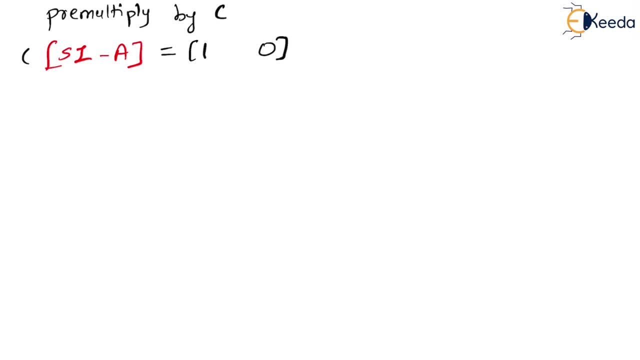 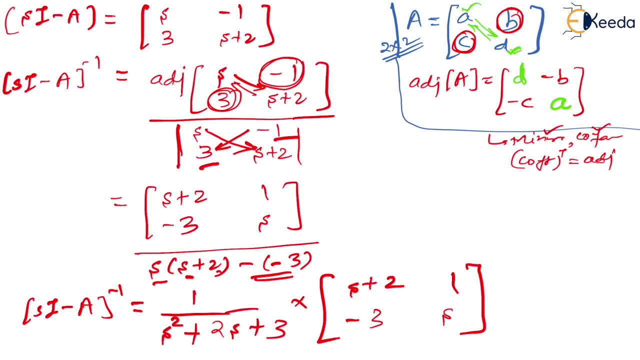 Because Y equal to CX plus DU. Whatever is there with X in Y equation, that is nothing but C. So this is C. So you have got this one zero And S- I minus A. you have already got What is that? 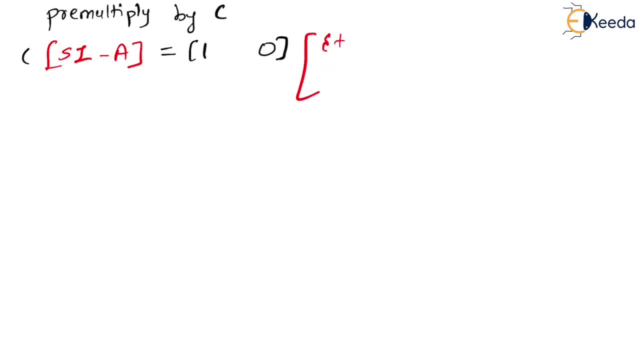 It is going to be S plus 2, 1 minus 3S, So S plus 2, 1 minus 3 and S. Am I right? Yes, definitely. Now you just simply multiply, You just simply apply the matrix multiplication. 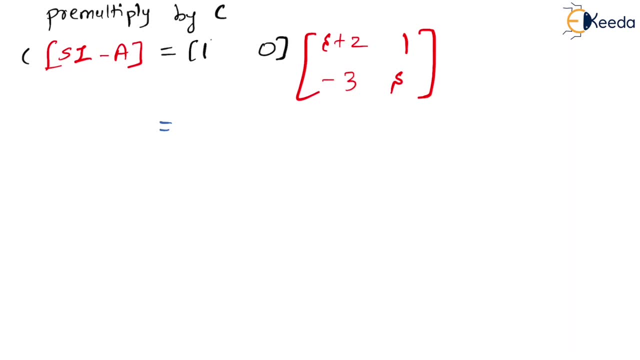 So to apply that, what do we do here? So, if you apply that, what do we do? Yes, 1 into this, 1 into S plus 2.. What is that going to be, By the way? by the way, by the way, 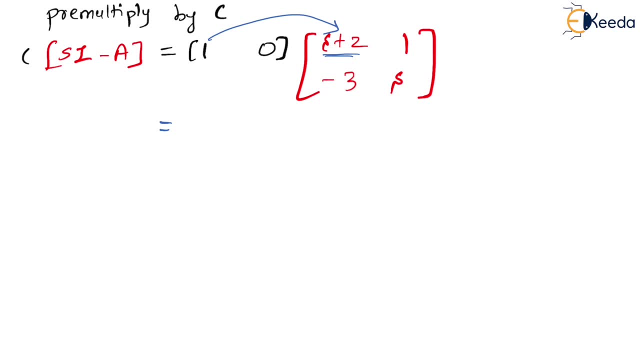 You also have to do this. You also have to do this. You also have this term. right, You also have this one. What do you say? You also have this one multiplied by determinant. What is the determinant Determinant is S squared plus 2S plus 3.. 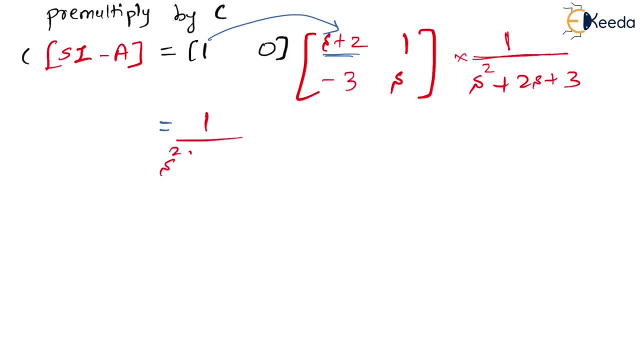 You also have this one right: 1 upon S plus 2.. So let me have this 1 upon S squared plus 2S plus 3 here. There is no problem. Now let me multiply. Let me do the matrix multiplication. 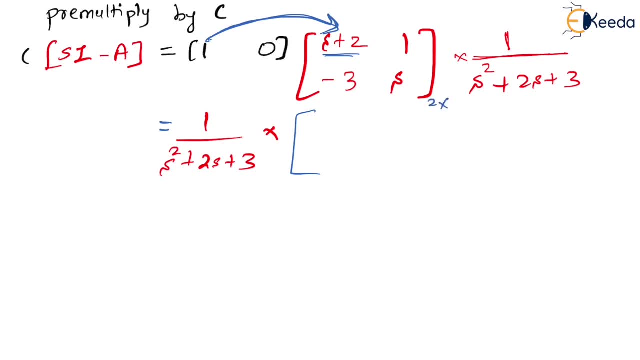 So what is going to be S 1 into this one, Because it is row by column. By the way, it is just a row. Just see here: This is 2 cross, 2 matrix, And this is the. it has 1 row and 2 columns. 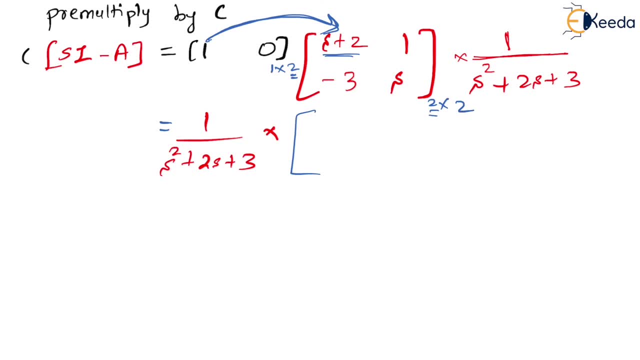 So this is going to be 1 cross 2.. So, yes, definitely 2, 2 is common. So matrix multiplication is possible or not? Yes, And this 1 cross 2 is going to be what It is going to be, your, this one. 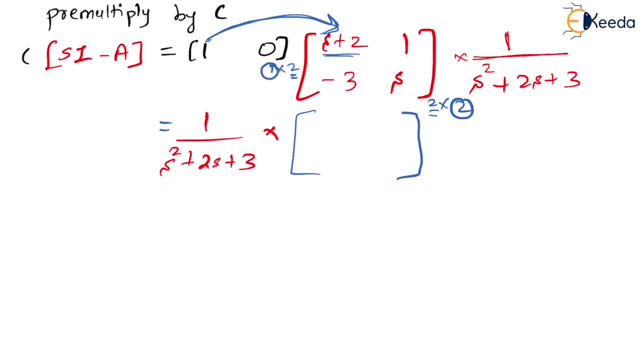 So it is going to be 1 cross 2.. So let me have this as 1 cross 2 matrix. 1 cross 2 matrix. So only 1 row is going to be there Right, 1 row and 2 columns. 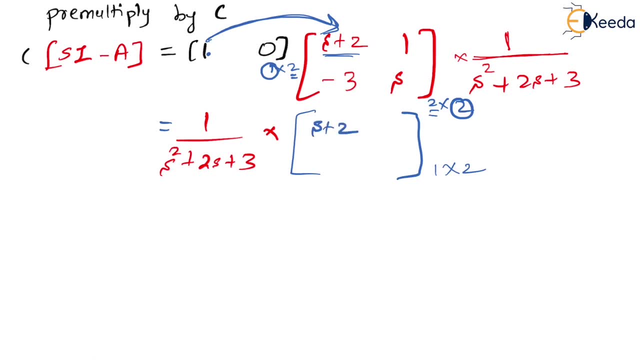 So 1 into this is S plus 2.. Similarly, 0 into 0 into minus 3 is going to be 0. So plus 0, plus 0 into, if you see again this, 1 into 1 is 1.. 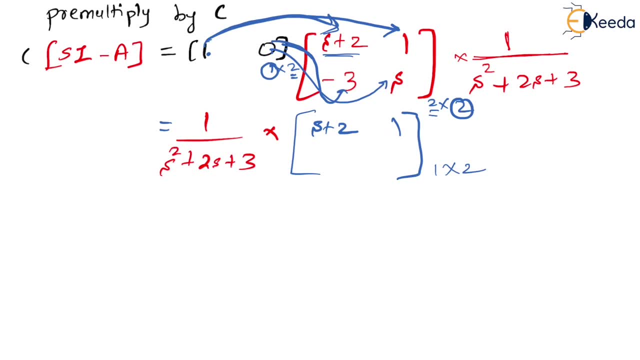 So, and this 0 into 3. S is going to be again 0. So it is S plus 2 and 1.. Right Now, this is nothing but 3 into S minus A. Now you need to have B also. 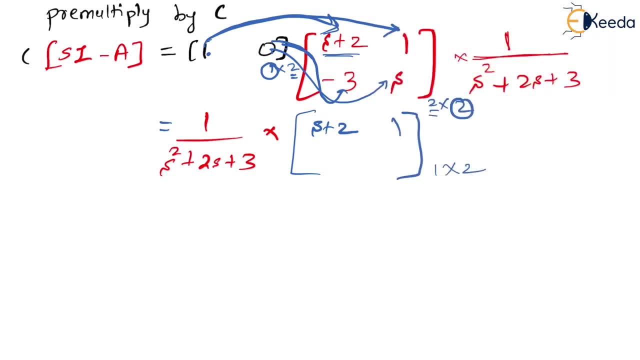 So let us post multiply by B. Let me post multiply by B. So if I do this, post multiplication by B, what do I get? here is C into S I minus A. inverse is already there, but this is inverse, not S I minus A. 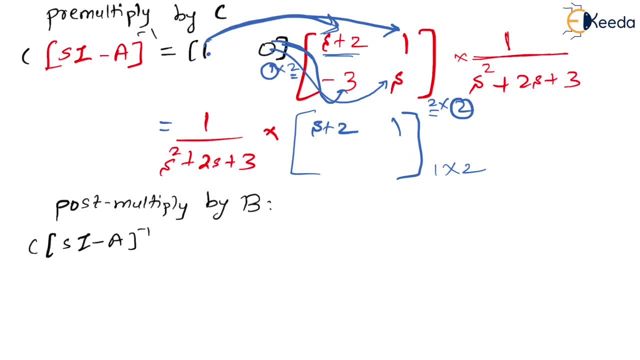 This is inverse right C into S, I minus A. already I have multiplied by B, So what is B here? Yes, If I multiply by B, then what do I get? 1, 2S squared plus 2S plus 3.. 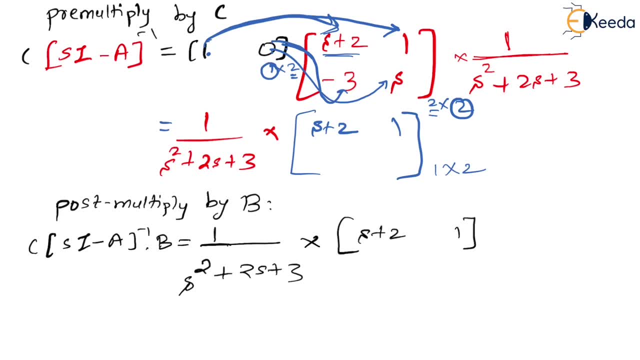 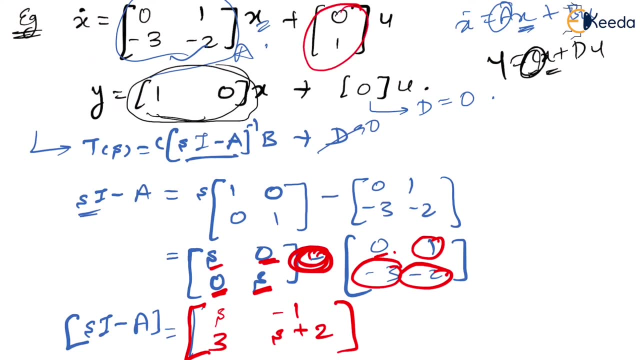 Right, Multiply by this one S plus 2, and this 1 is going to be there. Yes, If I multiply this by B, so it is going to be what is B here? Yes, B is going to be 1, by is going to be 0, 1.. 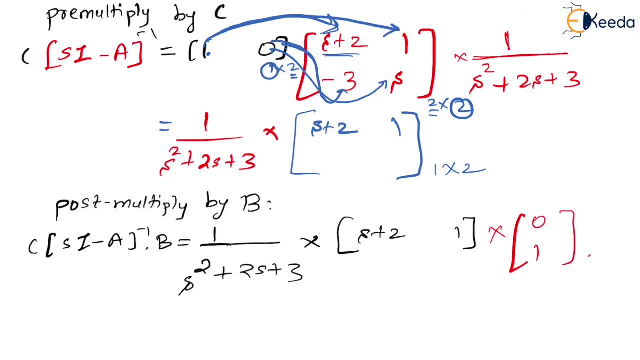 So it is going to be 0, 1.. So if you just see here, what do you get At the end is going to be: this is 1 upon S squared plus 2S plus 3, right. 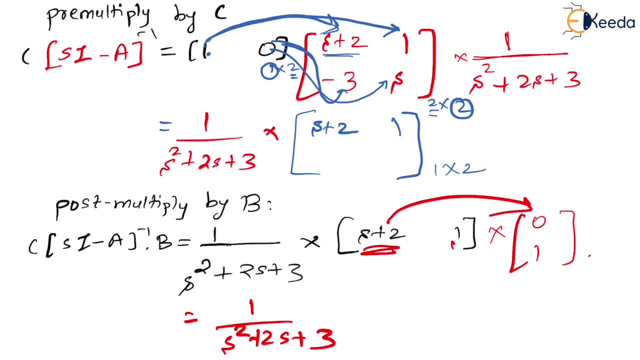 At the end. if you see, what do I get? is this S plus 2 into 0 is 0,, 1 into 1 is 1, right, Because this is going to be 2 cross 1 matrix and this is going to be. what do you say? 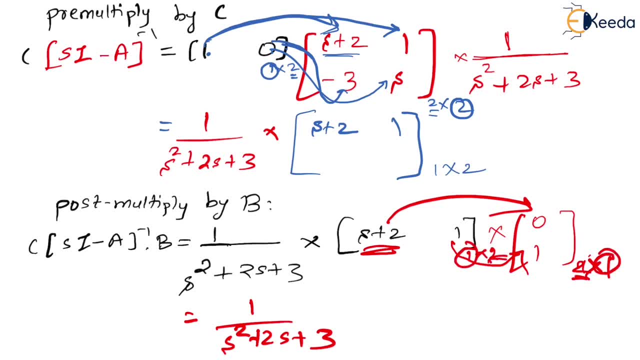 1 cross 2 matrix right. So 2, 2 is going to be common and this 1 and 1 are going to be the common. So this is going to be 1 only. So at the end it is 1 only. 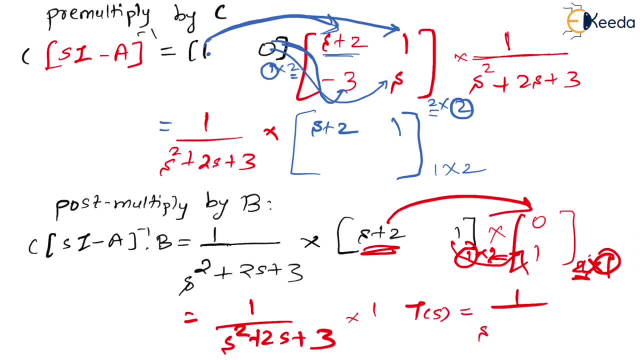 So what is the transformation that you get here? Transformation that you have got is 1.. 1 upon S squared plus 2S plus 3.. I know I have gone from a very, very basic level, but, yes, it is going to be very, very important. 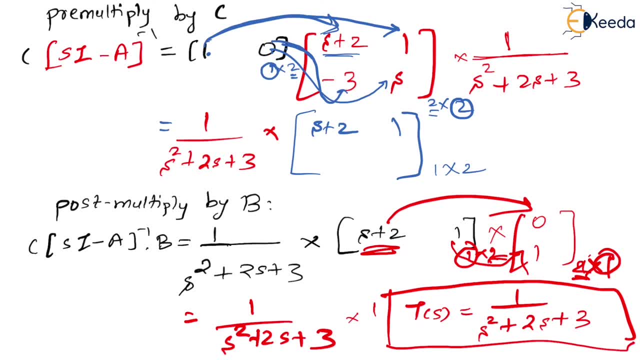 because I need to take care of each and every student, right, Anyway? so the transformation that you have got is nothing but 1 upon S squared plus 2S plus 3.. So this is all about finding a transformation from a state space model. Thank you, Thank you.